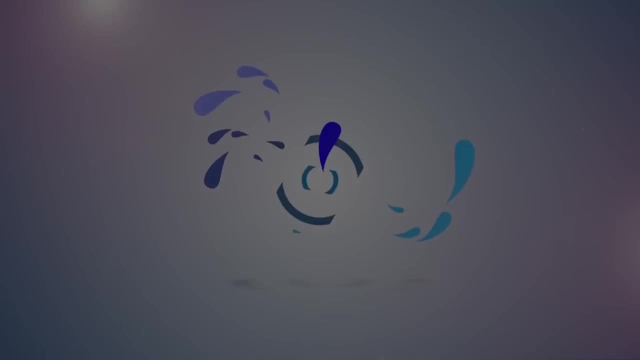 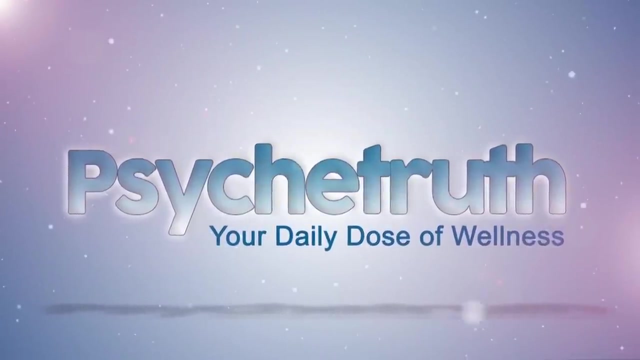 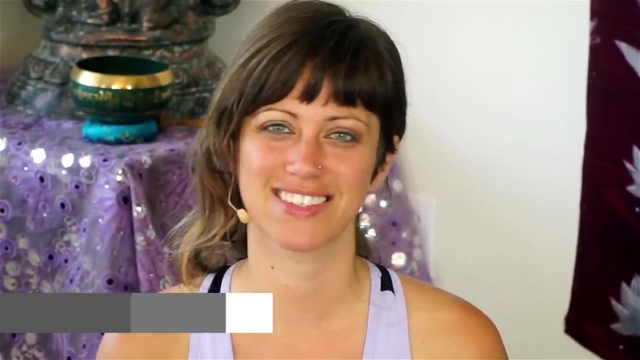 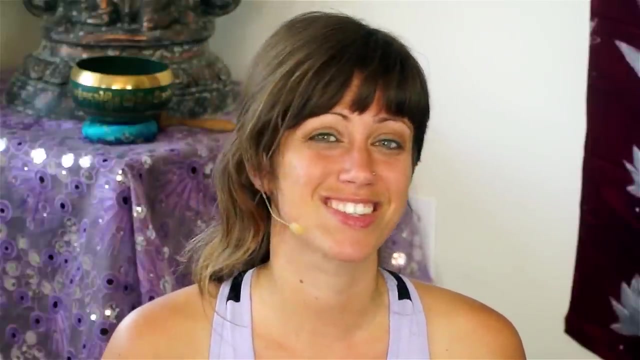 New videos every day: Psyche, Truth, Life, Wisdom. Hi, I'm Jen Hillman. Thanks for joining me today. This is part of my series of Yoga for Dummies. This is just a series geared towards people who are absolute beginners. 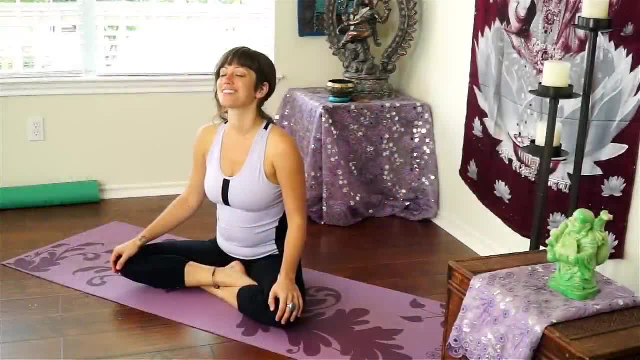 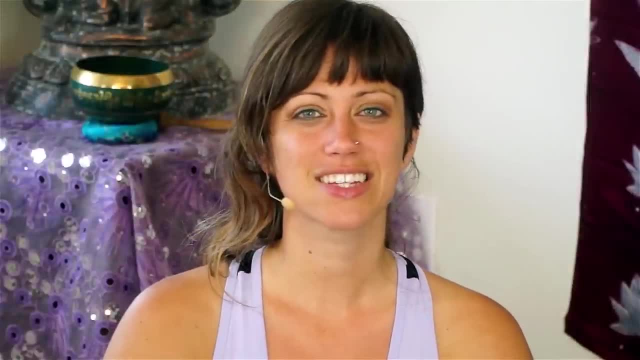 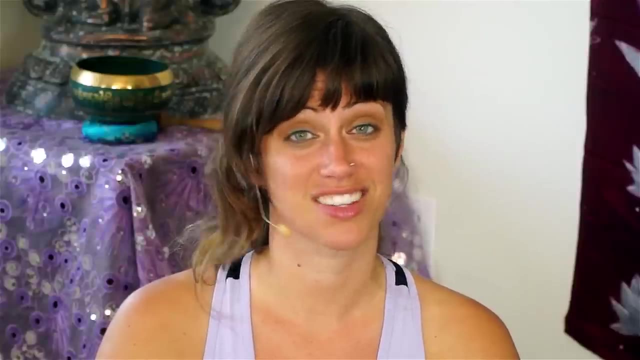 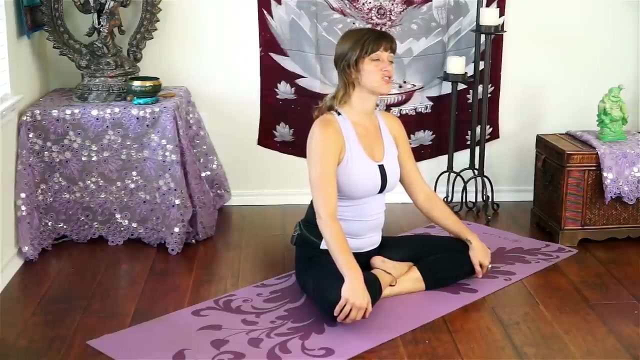 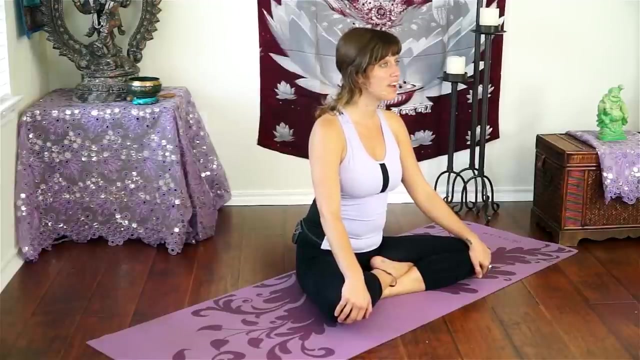 Maybe you've never done yoga before. This is the series for you, So thanks for joining me today, And today's video is geared towards helping you achieve a state of relaxation. Yoga has so many benefits, And stress relief and relaxation are some of the main and primary benefits that you will get from a regular and steady yoga practice. 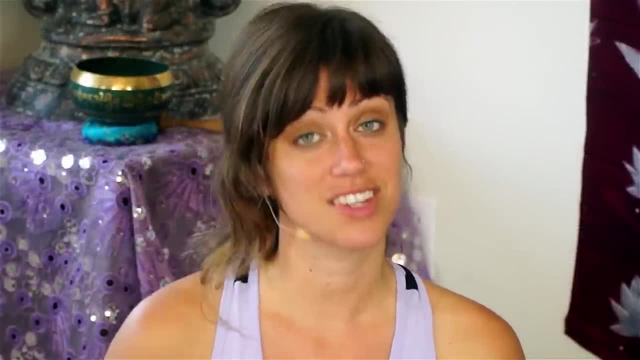 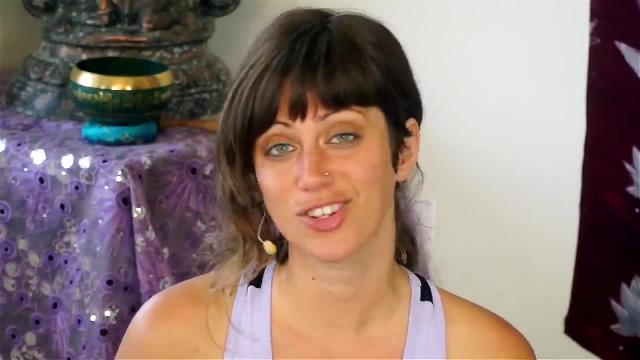 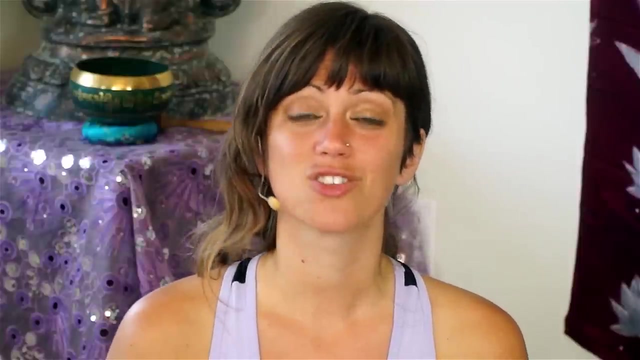 So we are going to get started sitting down So if you have a yoga mat, you can roll it out. If not, just practice right on the floor right where you are And go ahead and favorite This video so you can come back and watch it any time you're feeling stressed out and you need someone to help you relax. 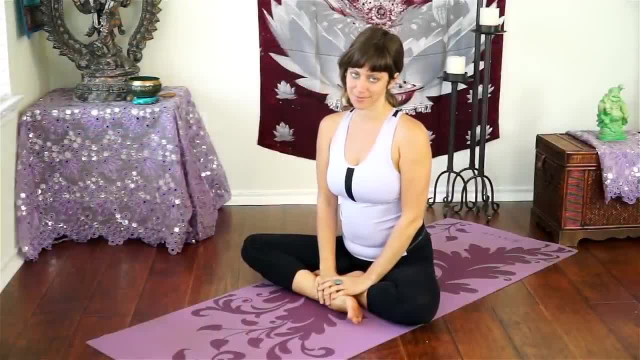 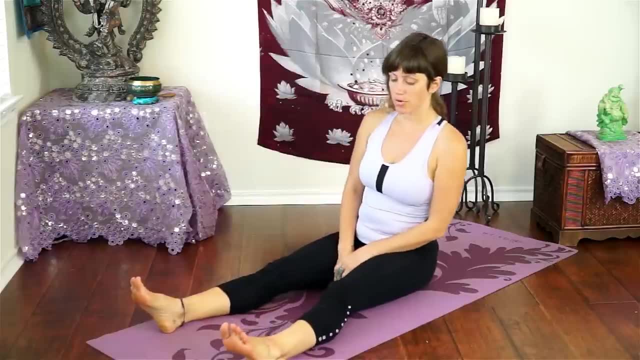 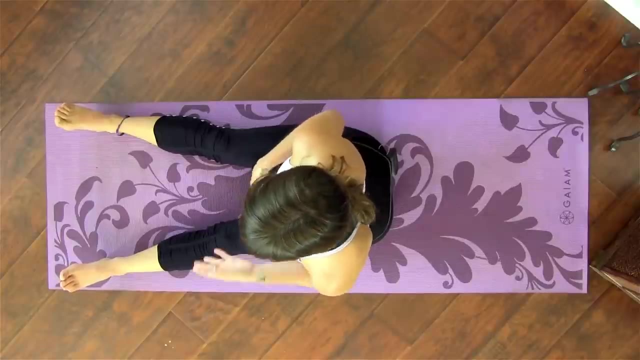 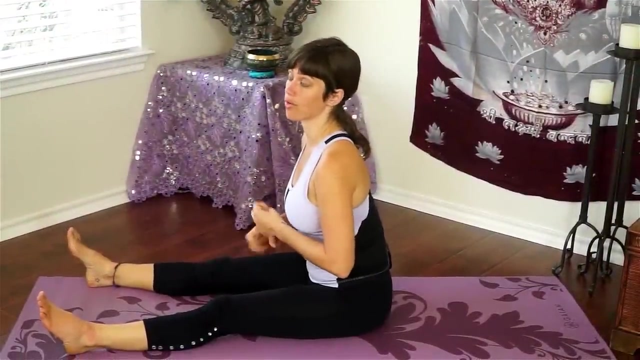 So, finding yourself in a comfortable seat, Go ahead and extend your legs forward. You can separate your feet a few inches apart, And if it's difficult for you to sit up straight with your legs extended, You can sit on a pillow or a folded up blanket. 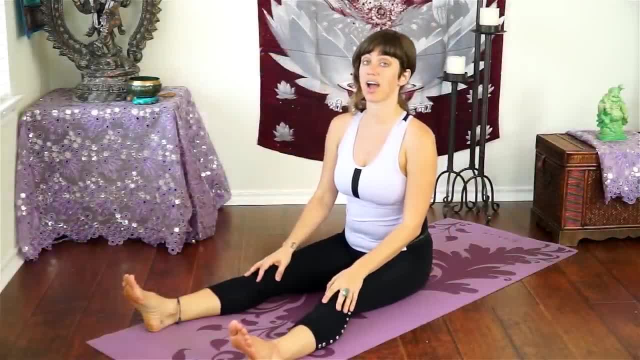 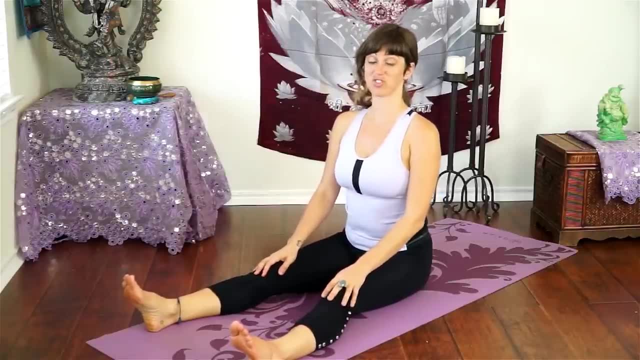 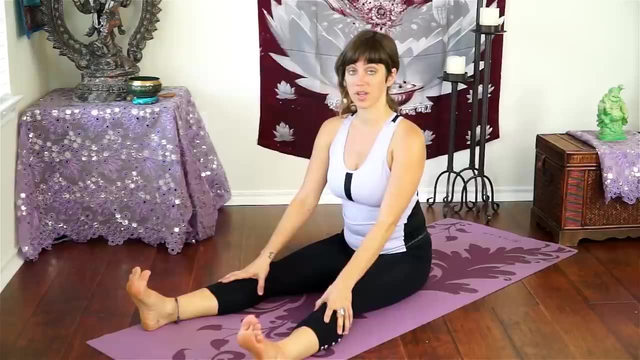 Anything that's going to help you lift your hips a little higher off the ground will make it easier to extend your legs forward and sit up with a straight spine. So, with your legs extended in front of you, we're just going to take a gentle forward fold here. 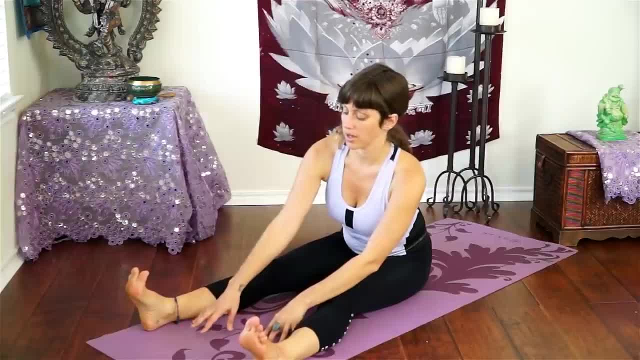 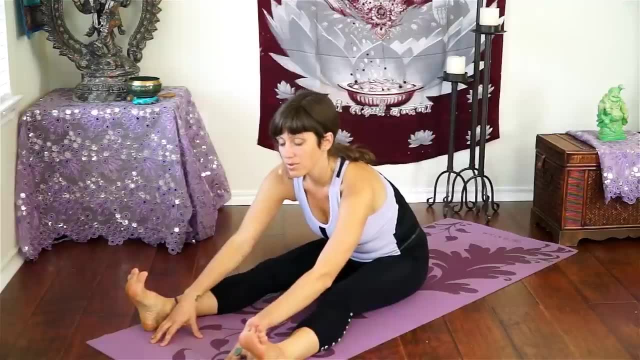 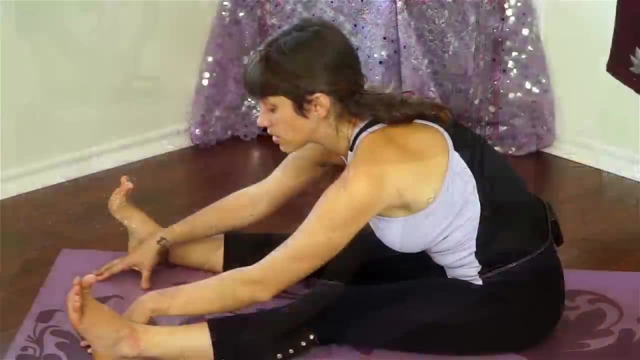 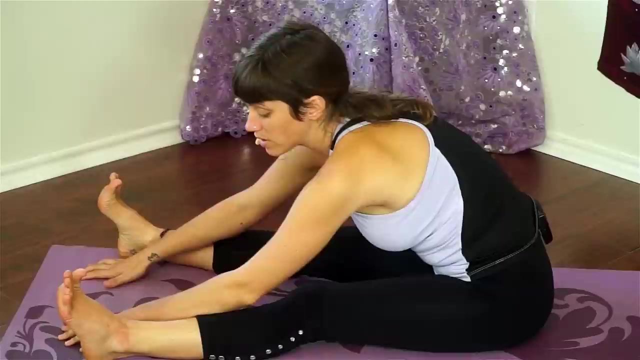 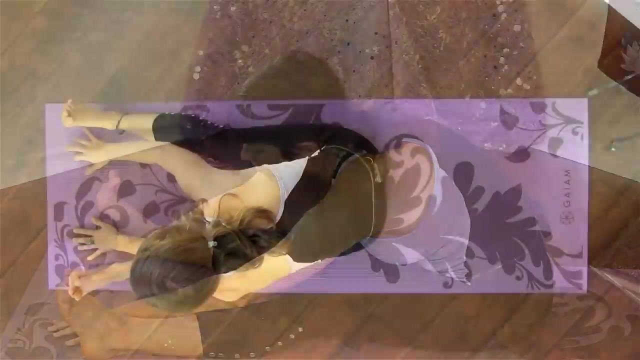 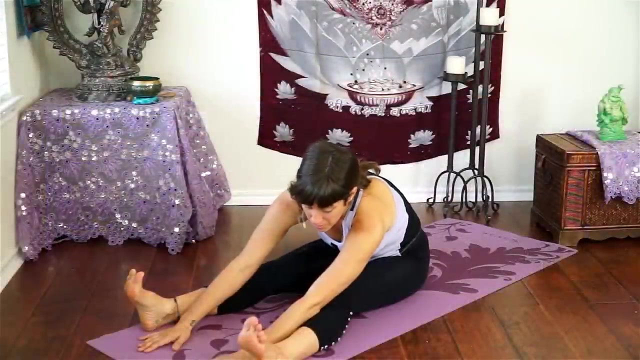 So just slowly start to walk your body forward and it's okay to shift from right to left. This will help to start to stretch out your spine and shift this stretch from your right leg To your left leg, And there's no rush here. 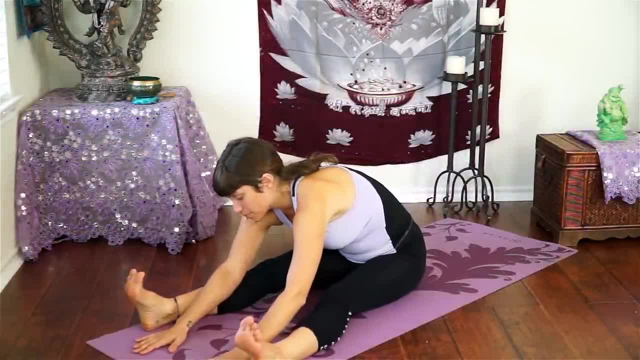 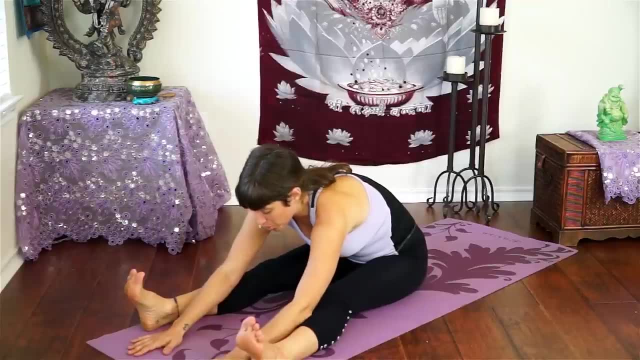 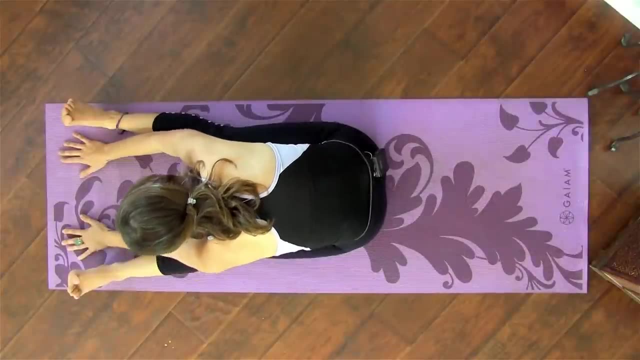 You can really take your time, Slowly, Gently Rocking your body From side to side, Slowly, Gently Rocking your body From side to side, Slowly, Gently Rocking your body From side to side. 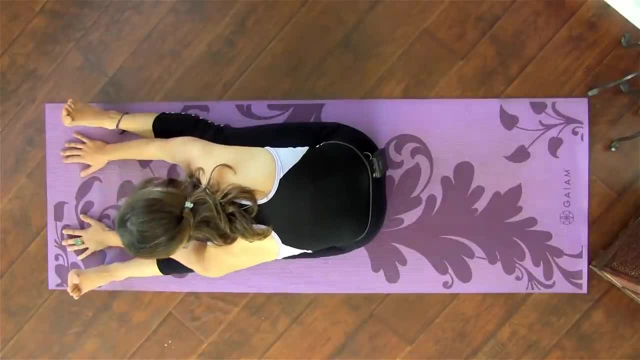 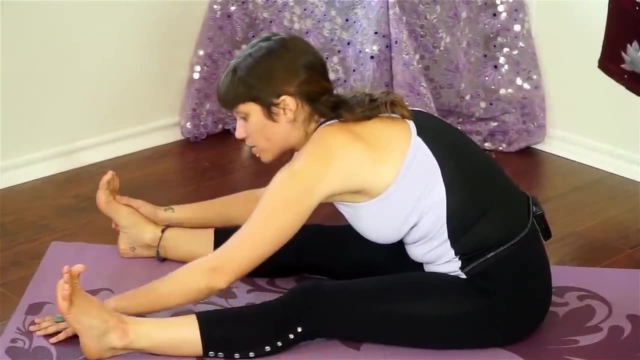 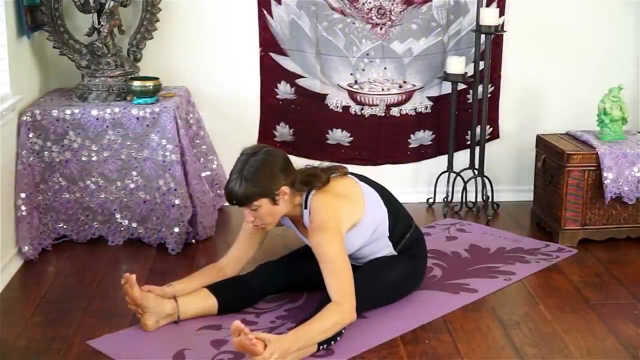 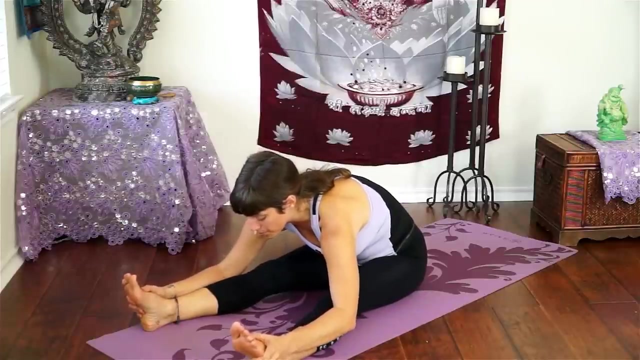 Gently Rocking your body From side to side. If you can reach your feet, you can hold on to them. This can help you slowly start to pull your body forward a little more. This can help you slowly start to pull your body forward a little more. 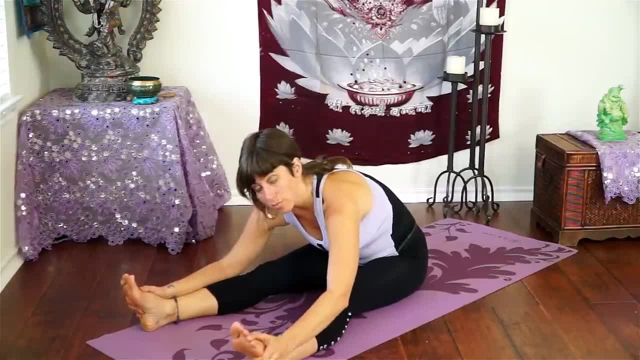 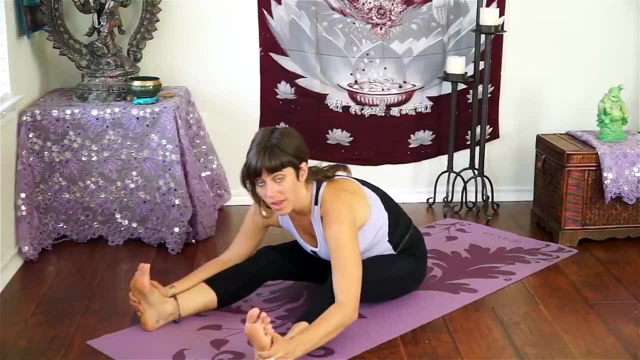 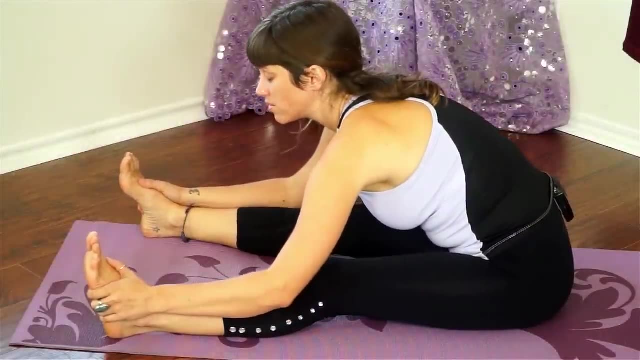 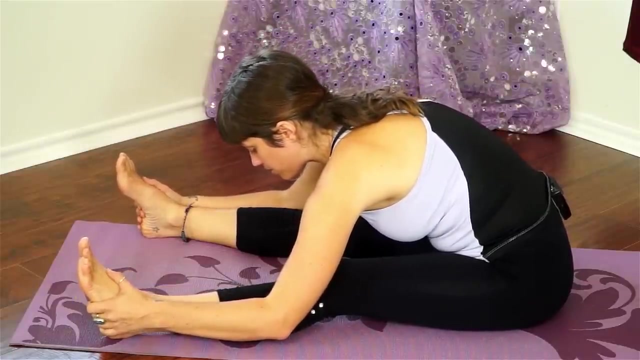 And if this is causing any strain or tension behind your knees, you can just bend your knees And that can help reduce the stress. So, wherever you are, just find your best stretch As we slowly come to stillness. As we slowly come to stillness. 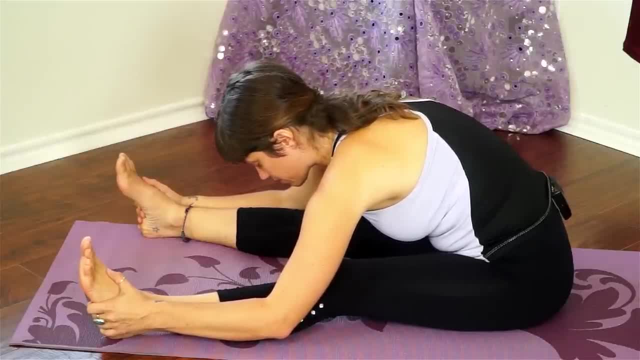 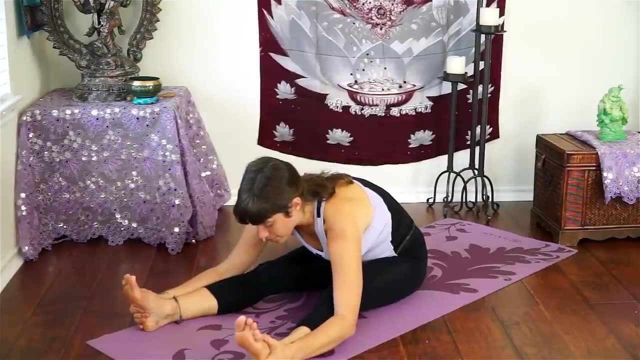 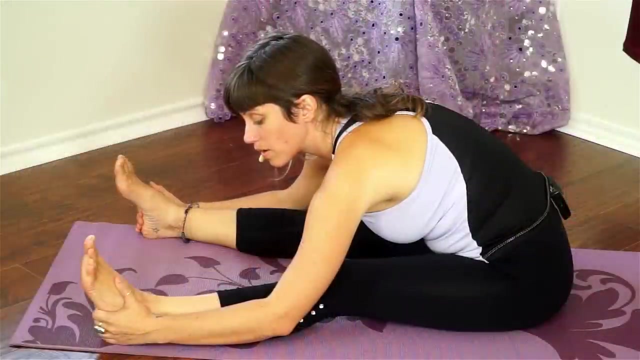 As we slowly come to stillness And let your head start to relax. So this video, Yoga for Relaxation, can be something really helpful to do before you go to bed at night. It can really slow down your nervous system And release tension in your body. 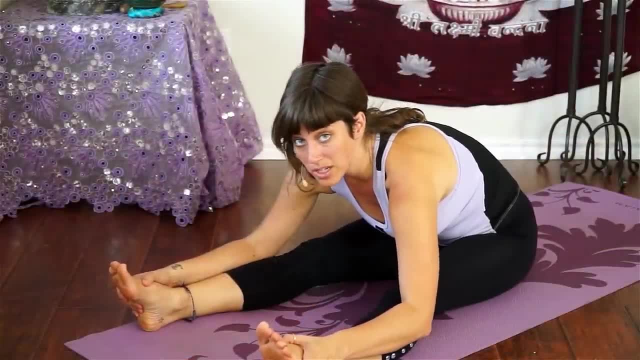 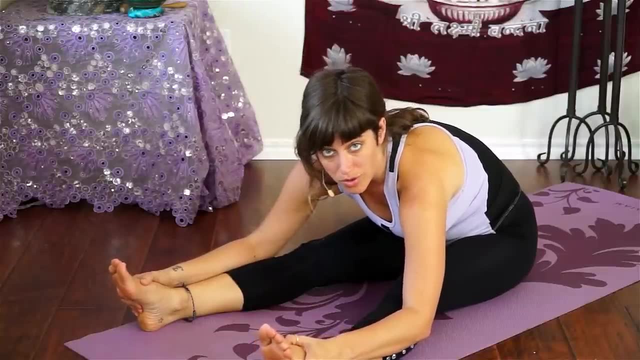 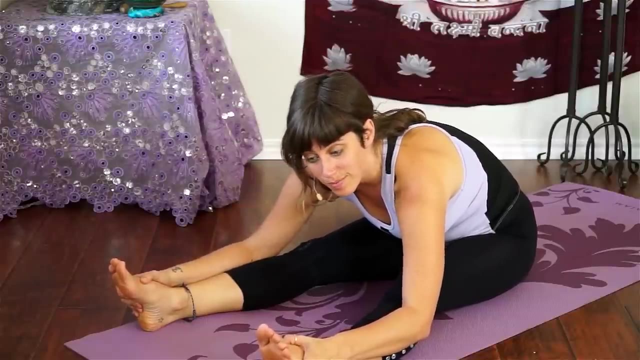 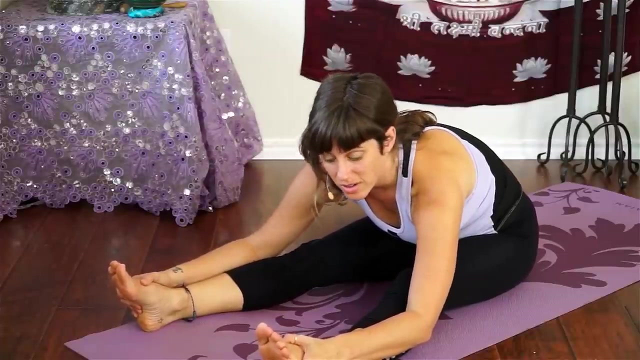 And so I wonder: do you guys have trouble, have trouble falling asleep? what is it that keeps you awake? is it hard to get comfortable, or is it your mind that won't let you rest? leave me your comments below and if you have any suggestions on ways that help you fall. 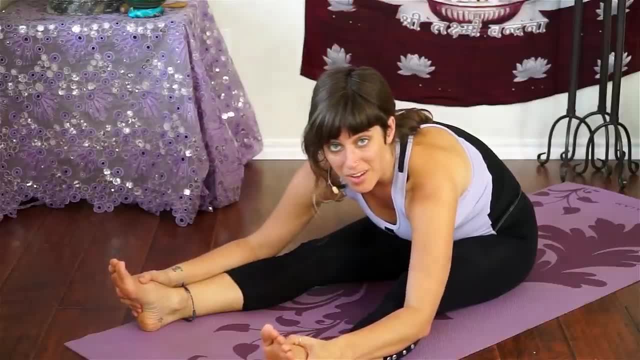 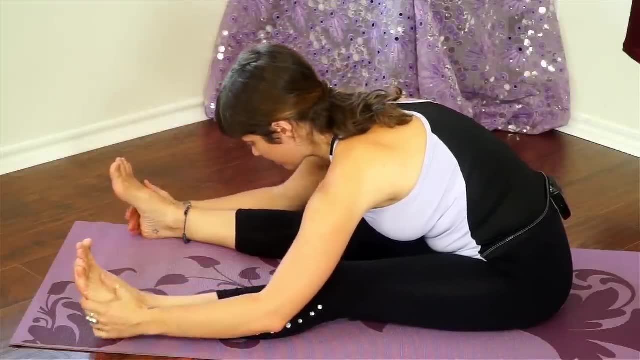 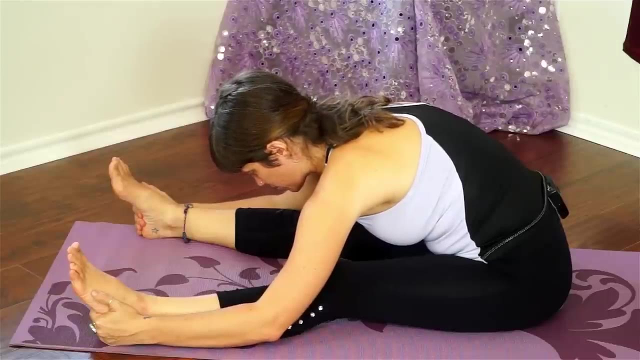 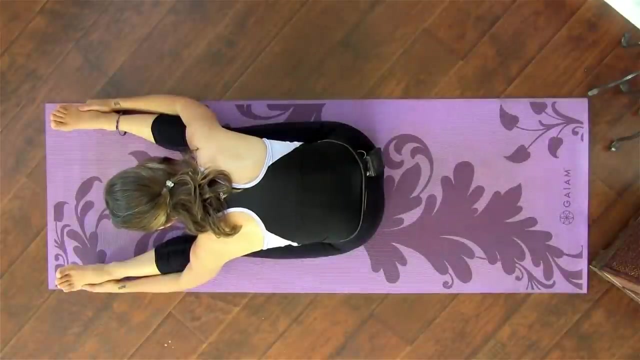 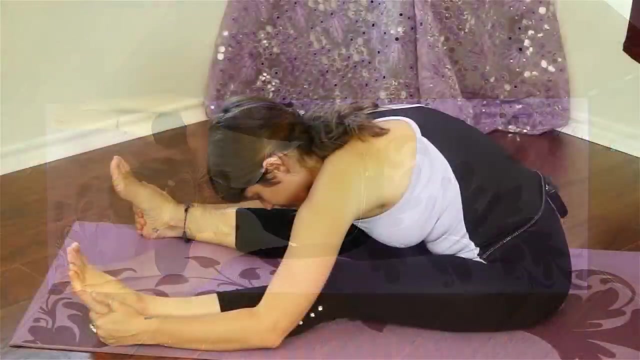 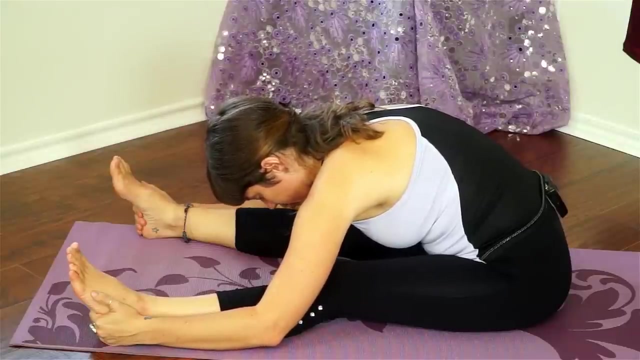 asleep. you can leave that below as well. we can help each other out, and after a few minutes in this stretch, you'll notice that your muscles are starting to feel a little more loose and relaxed, which might make it easier to stretch a little bit further. let your breath be slow and steady. 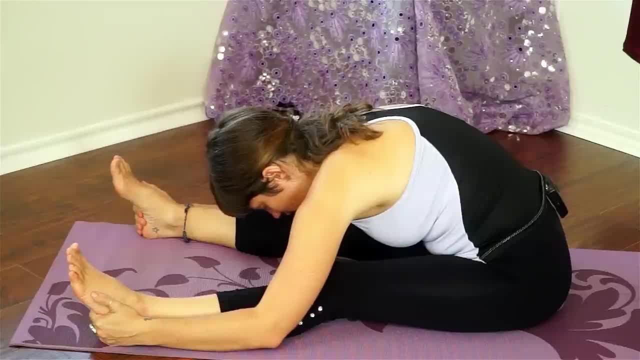 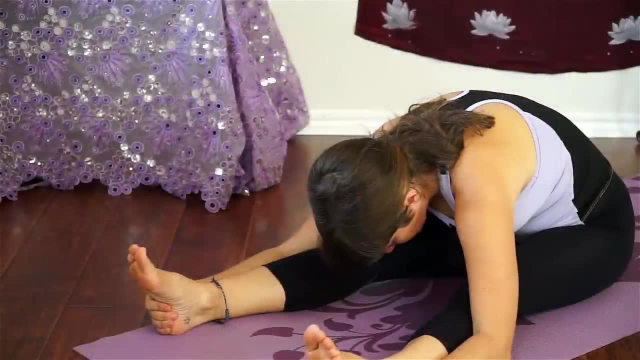 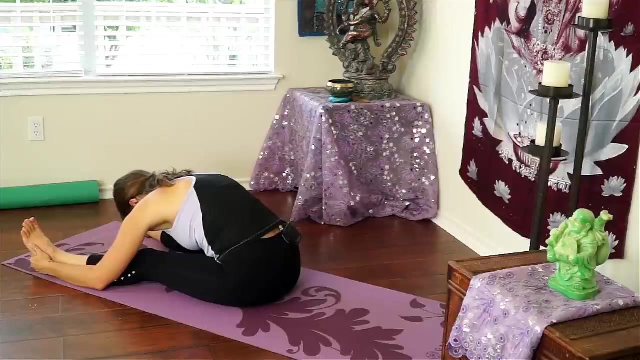 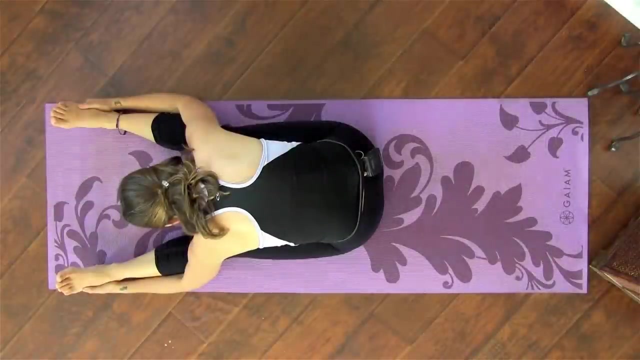 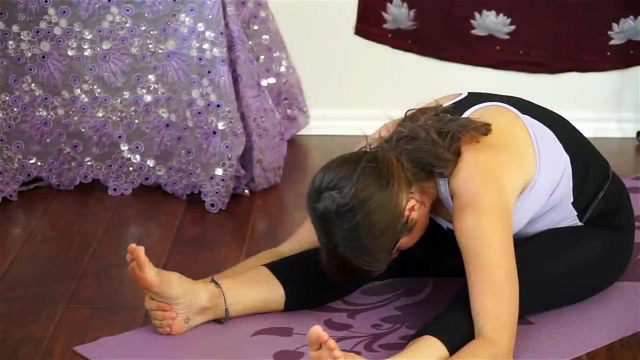 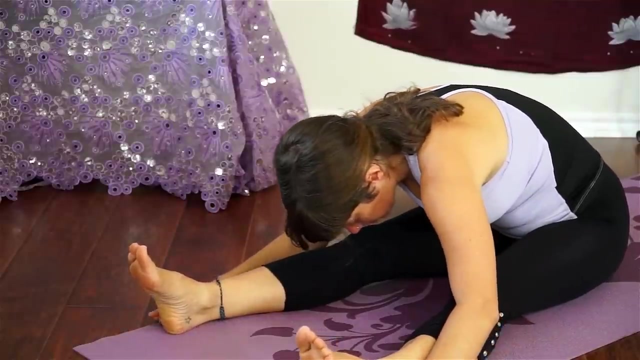 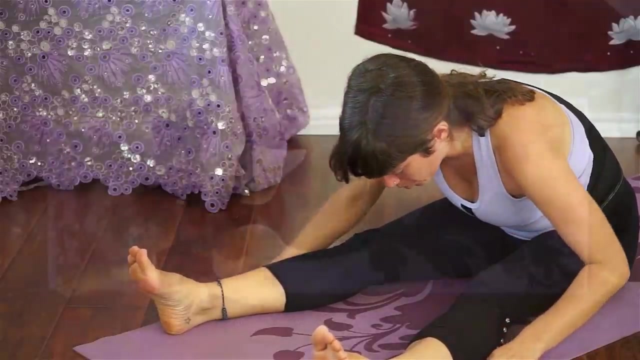 each deep breath helps you stretch a little further. so so you, being so so doing, do your Hare even本当 And then slowly, just as slowly as you came in, you start to gently rock back and forth, As you start to walk yourself back up. 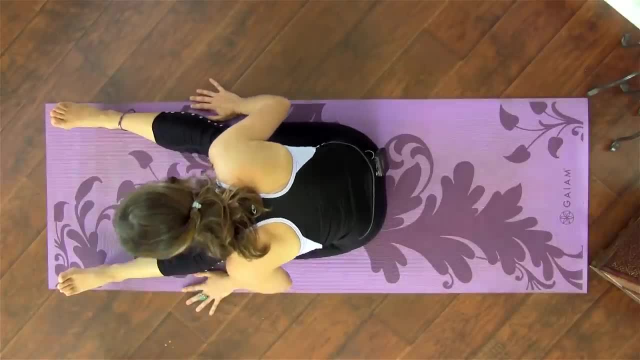 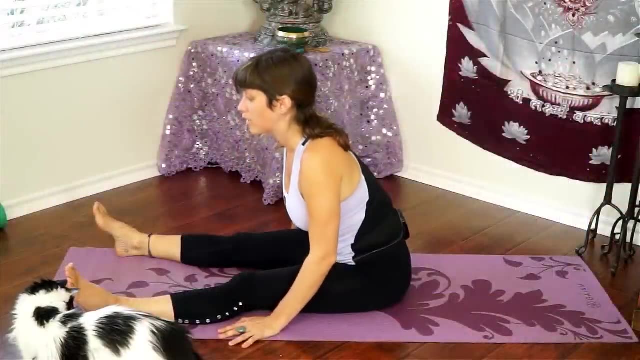 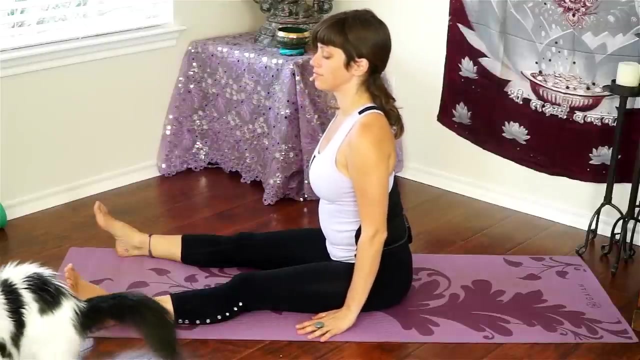 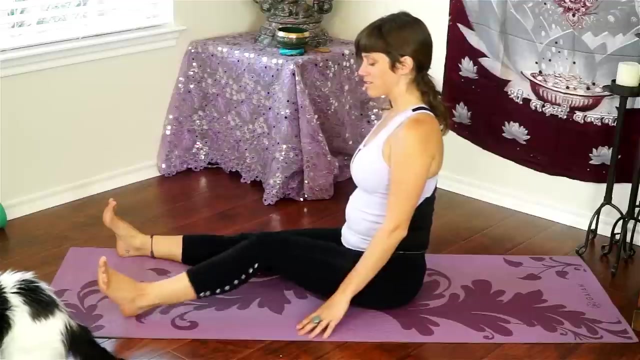 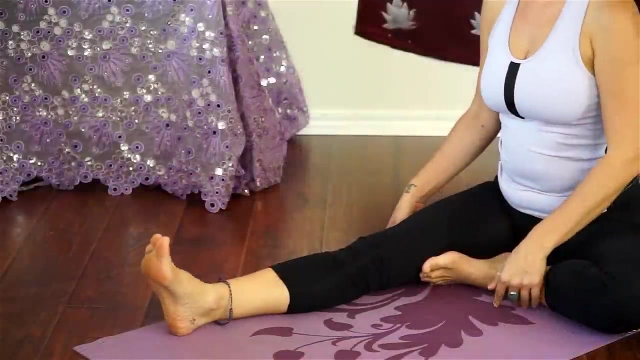 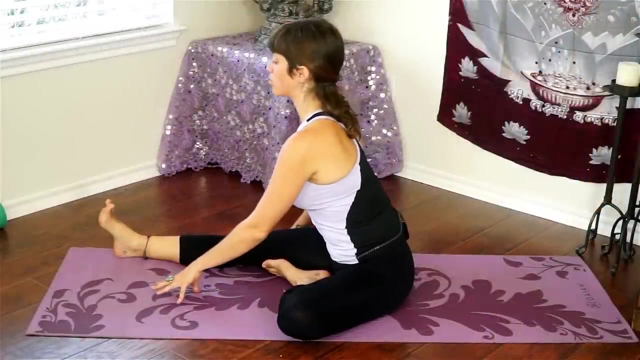 Rocking from side to side And you can use your hands to help you come all the way up And then bend your left knee so the sole of your foot comes to the inside of your right thigh. Now, with just your right leg extended, start to fold your body forward again. 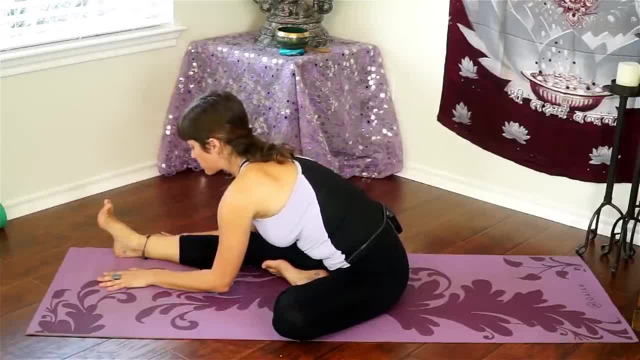 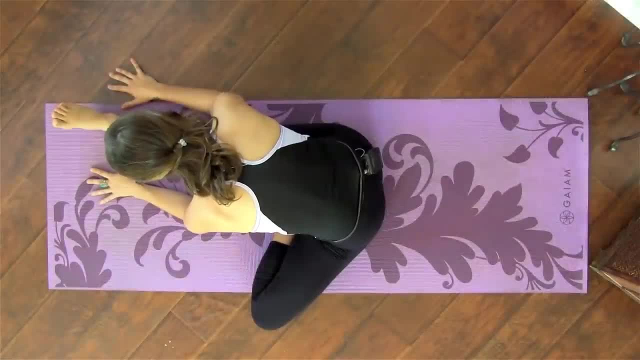 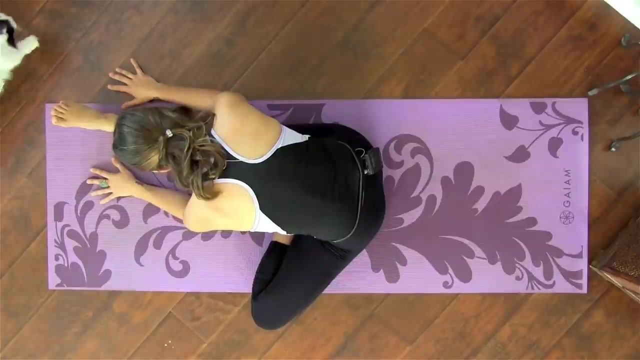 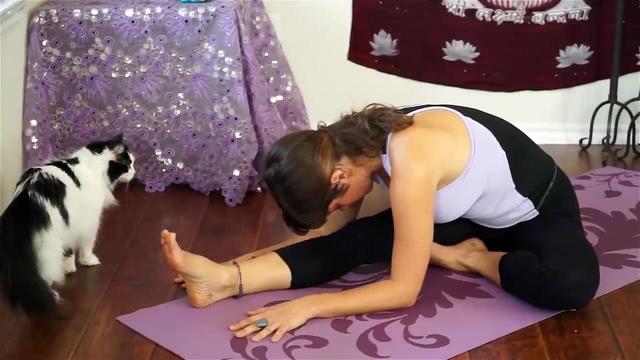 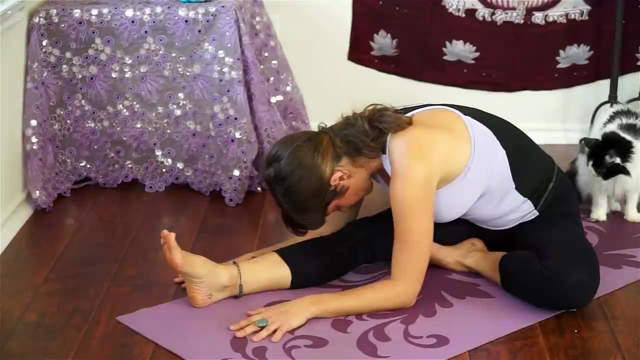 And notice how it feels different when you isolate just one leg. And remember, it's very relaxing: Relaxing to let the weight of your head drop down towards your leg, Creating a gentle stretch through your spine and your neck And just encouraging a sense of relaxation. 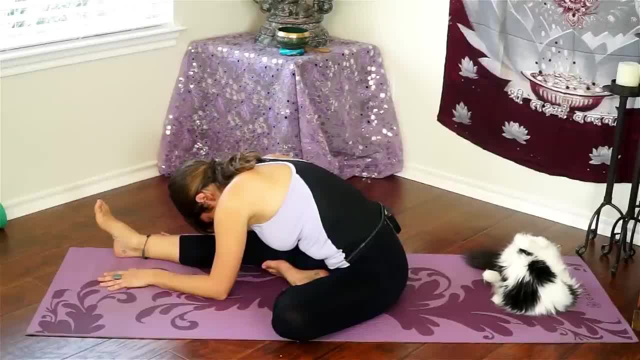 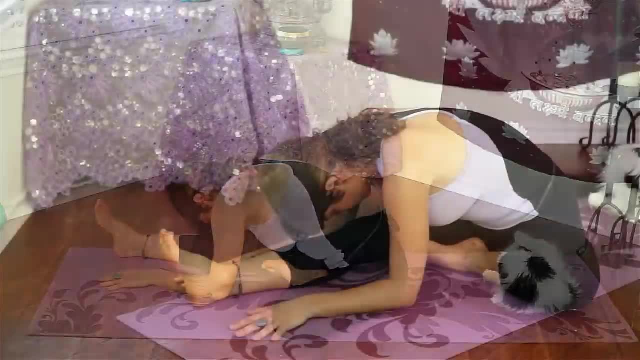 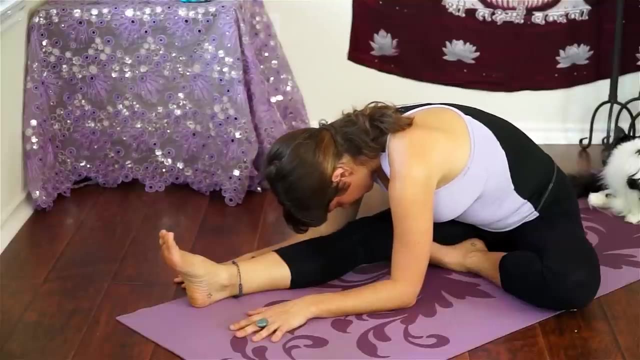 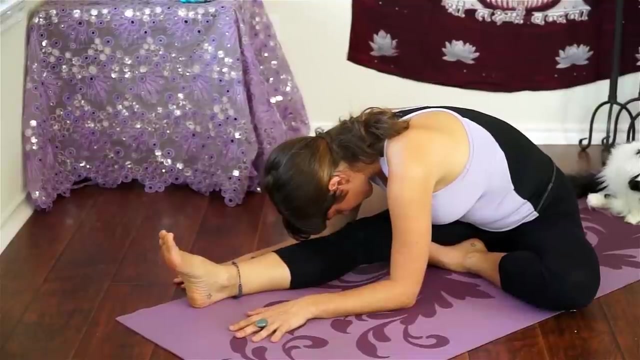 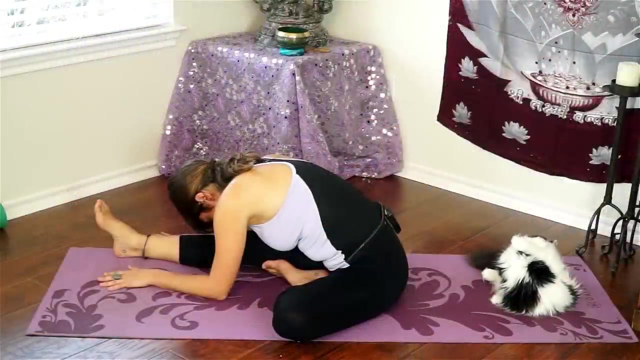 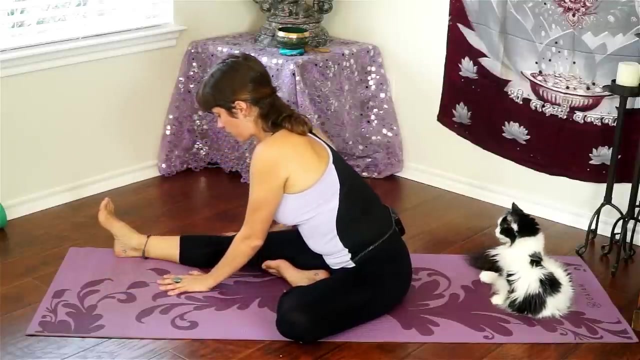 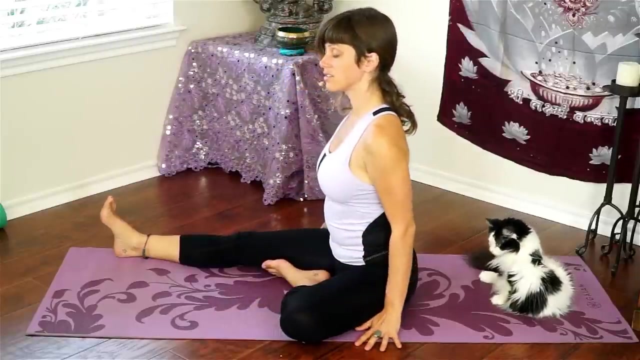 Relaxing into your stomach, tubing yourǐ with your right hand And slowly, a gentle swing it goes back up. Swing up your right heel, Push it up ği, And then again let's slowly start to come all the way up and change legs and bring. 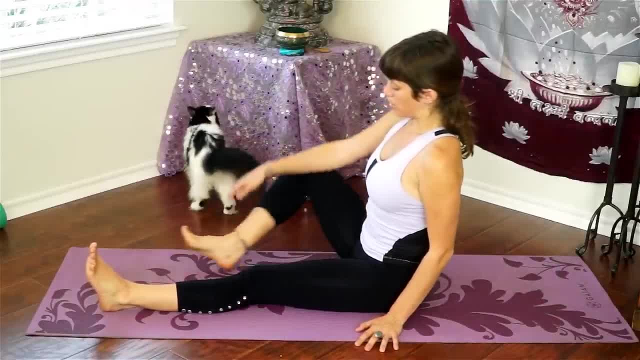 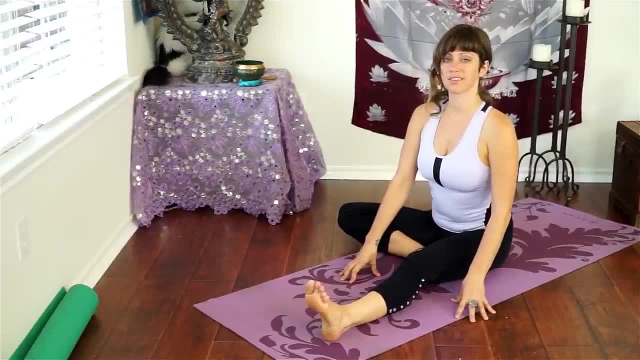 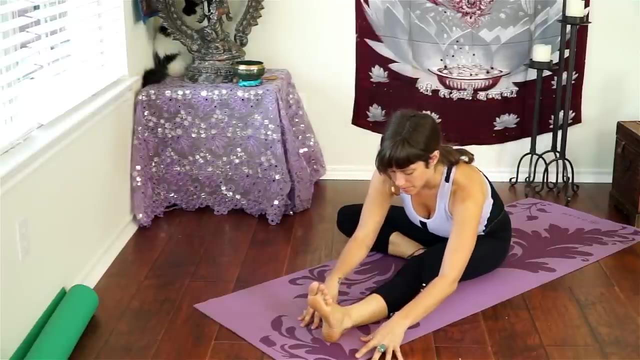 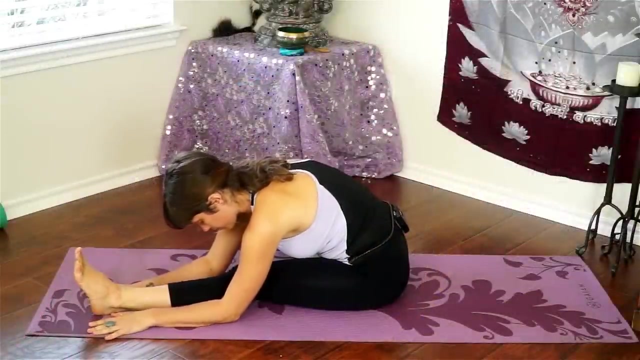 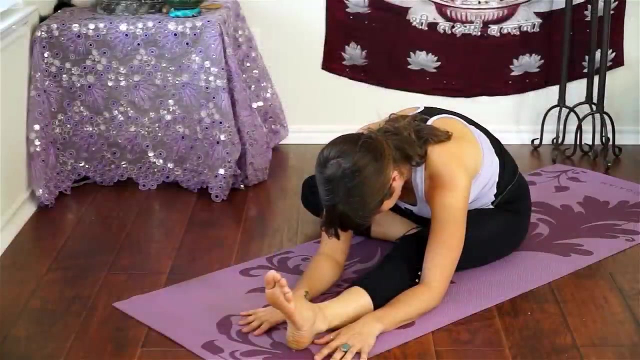 your left leg forward and bend your right knee and then again slowly start to walk your body forward towards your left leg and let the weight of your head relax, And if there's ever a stretch that feels too intense, just back off of it a little bit. 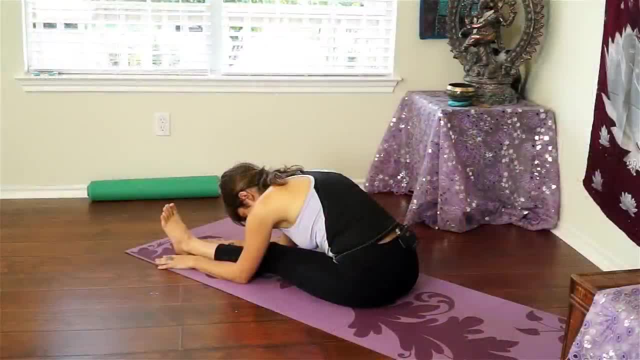 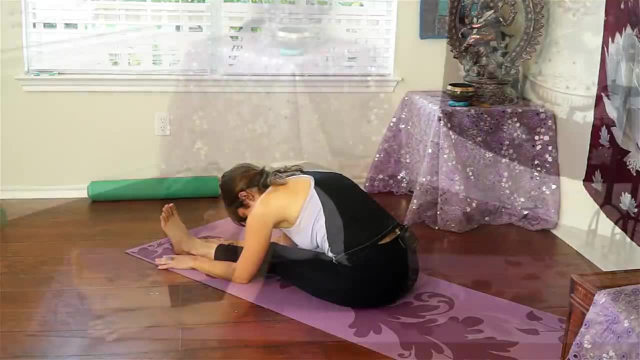 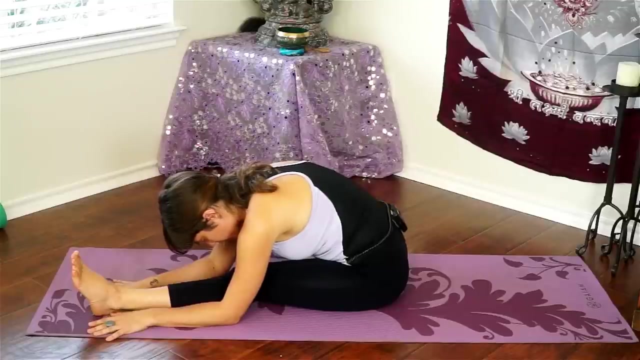 You don't have to go so deep. Okay, Back out to the place where it's not painful, it's not too intense. and remember, the more you can soften in your breath, the easier it will be to let your muscles relax. 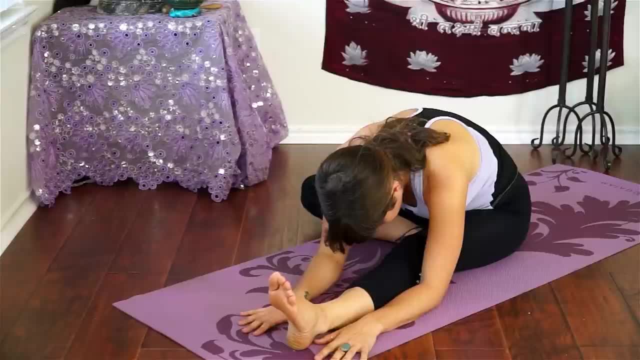 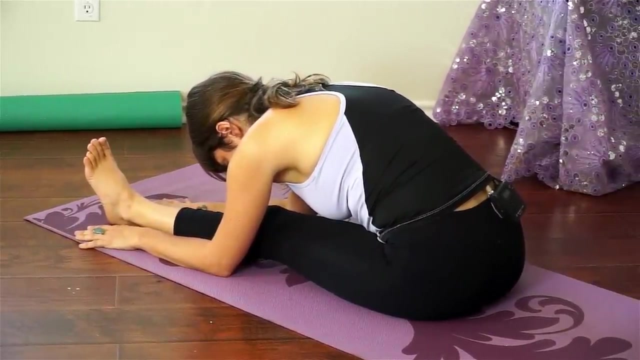 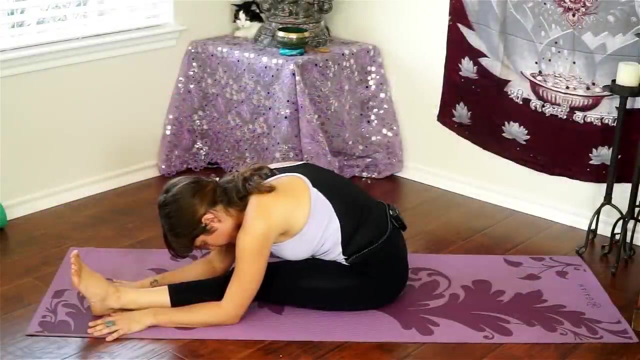 Okay, Good. And wherever you're noticing the most sensation, that's the indicator of where you're holding the most tension. So just use your breath to help you soften and invite those muscles to start to relax. Okay, Good. So now we're all very light, confident. 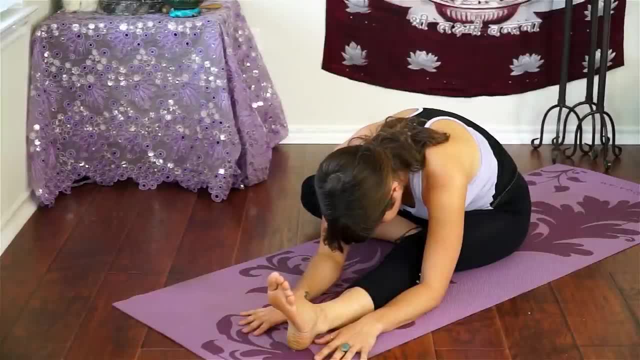 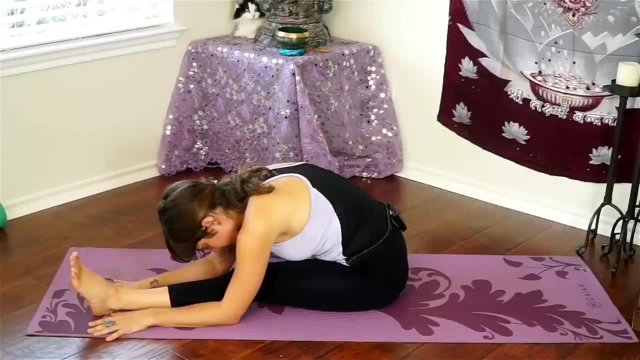 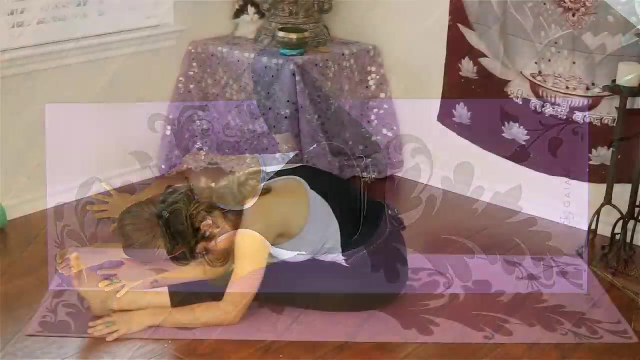 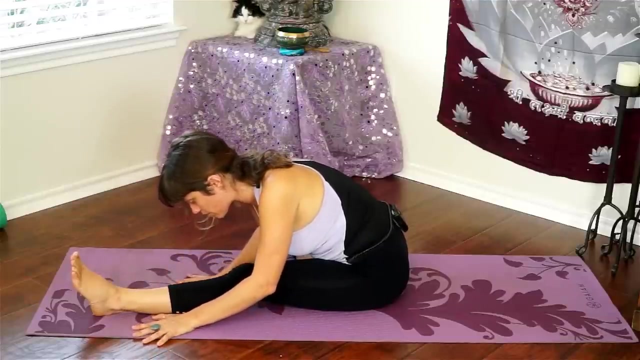 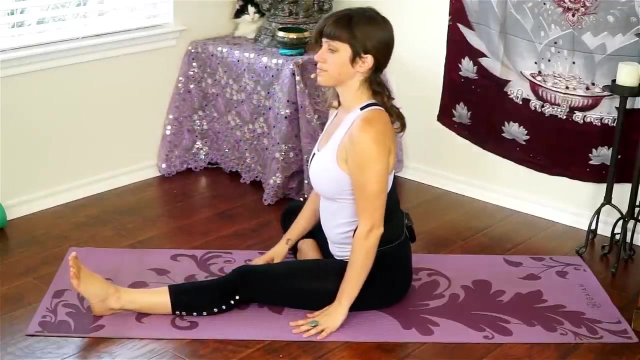 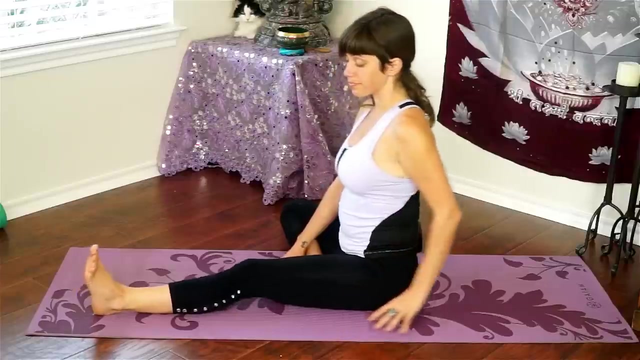 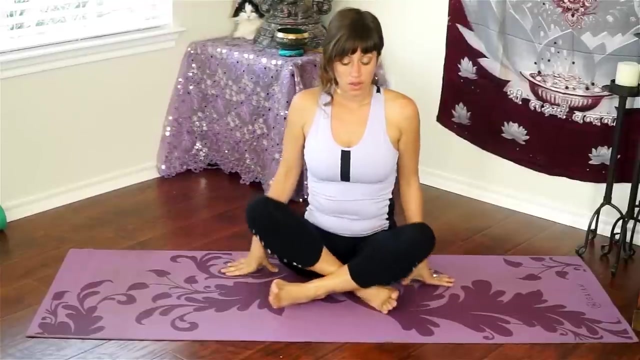 So just keep going. Ready Three, two, one, Relax, Pull over to one side, start to walk yourself back up. now we're going to take a wide legged stretch, so if you're using a yoga mat, turn your body so that you're facing the long edge of your mat. 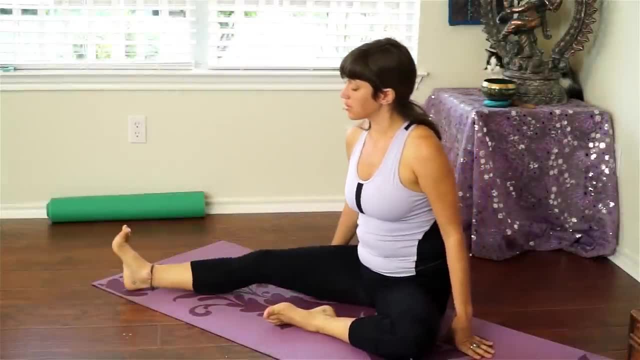 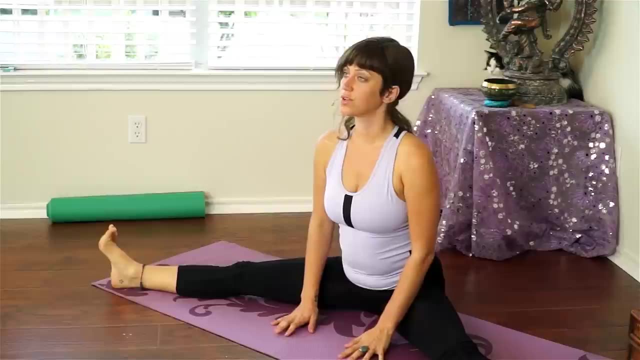 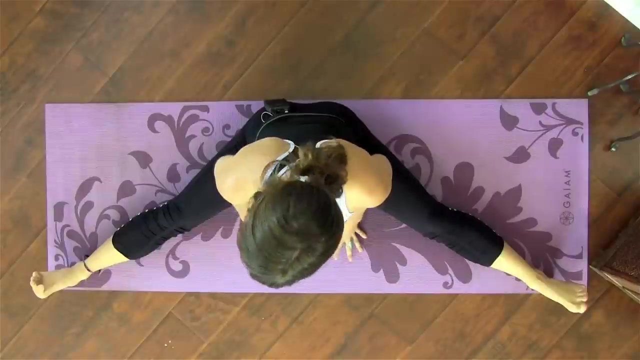 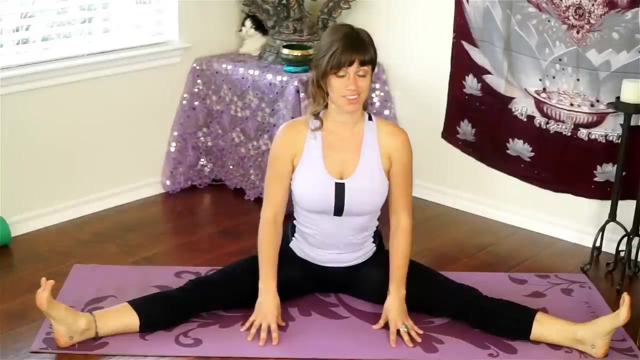 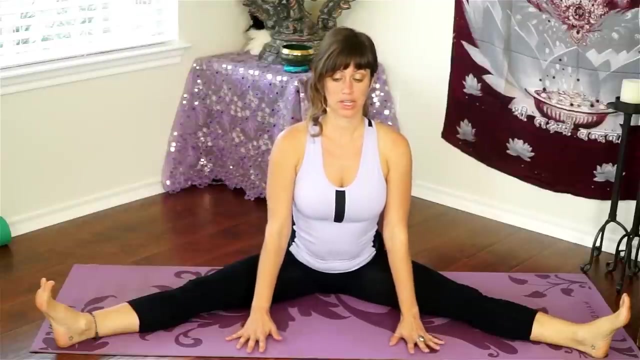 and extend your legs out to the sides. now you don't have to open your legs to your maximum stretch, just enough that you can feel a little stretch in your inner thighs, that's all. if this is enough stretch for you, you can plant your hands on the floor. 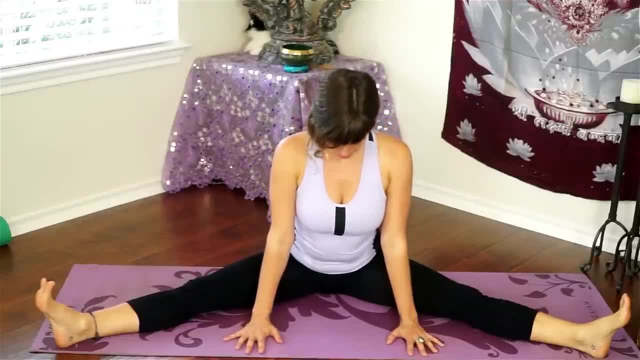 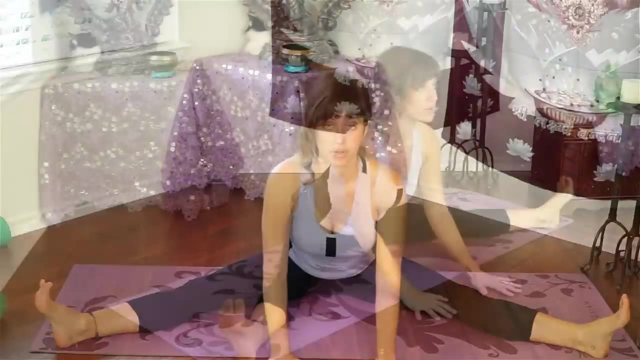 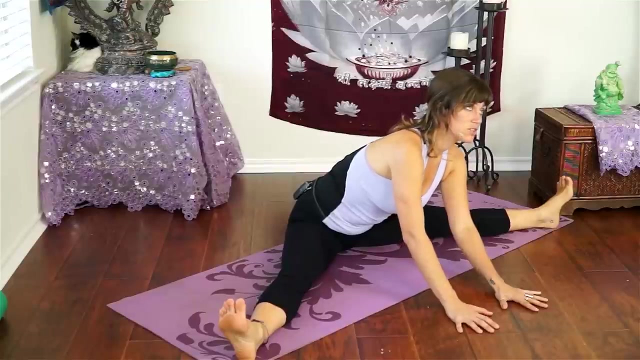 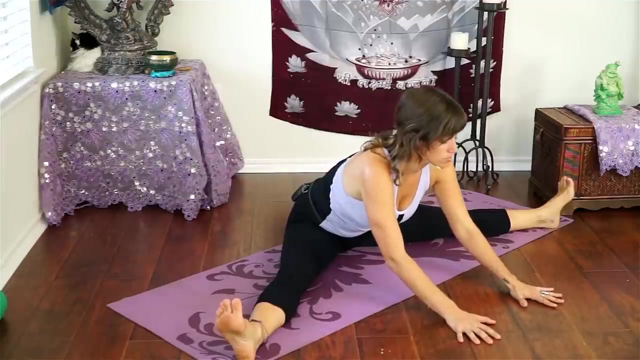 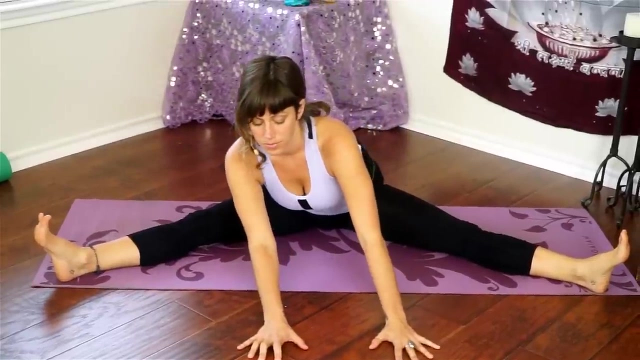 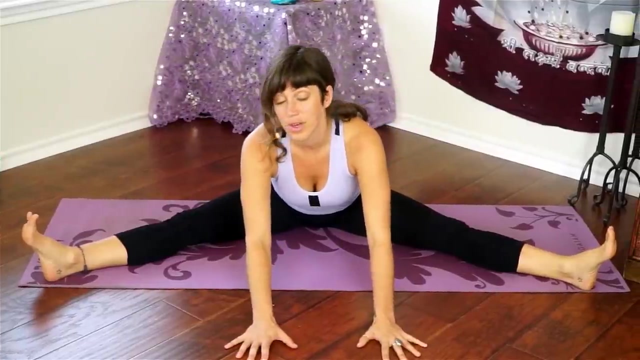 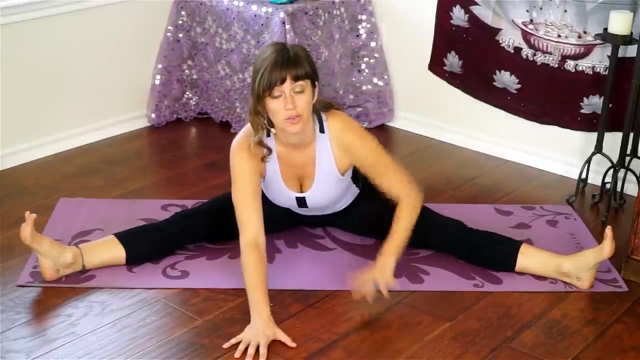 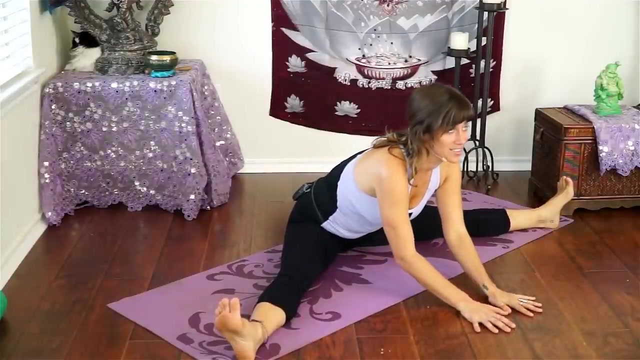 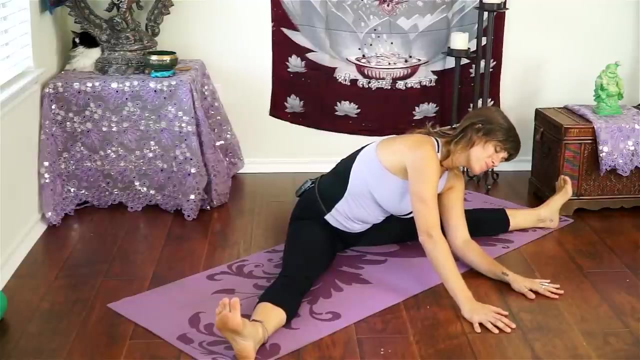 and just let your head start to relax. if you desire more sensation, slowly start to walk your body forward. you can shift from side to side. all that I ask is that you keep your toes pointing towards the sky. that's the safest place for your hips. other than that, you can stretch from one side to the other, or just stretch right. 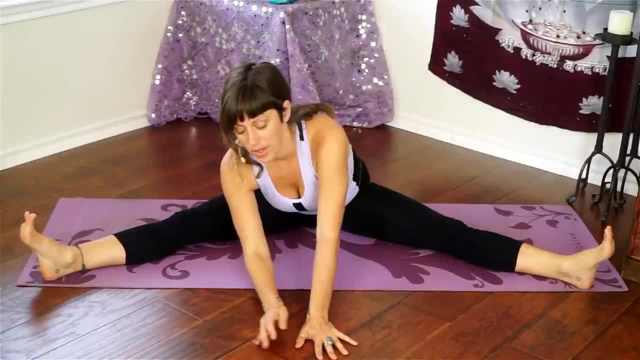 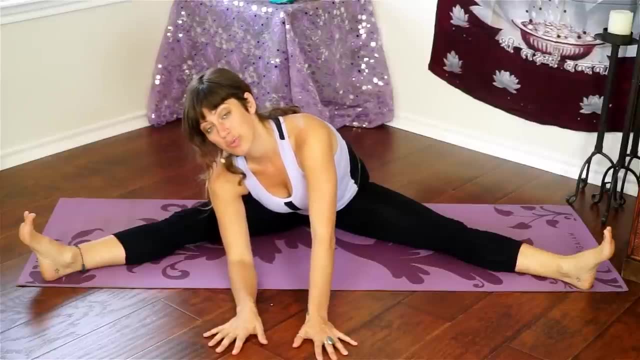 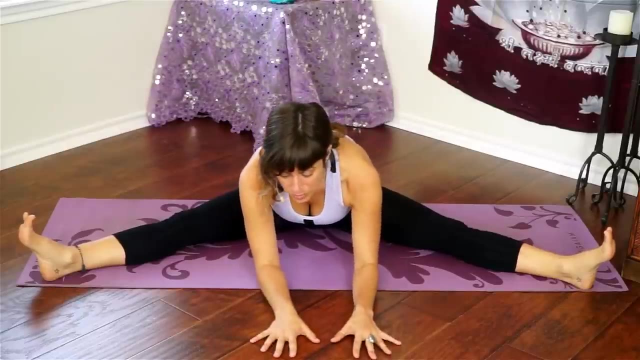 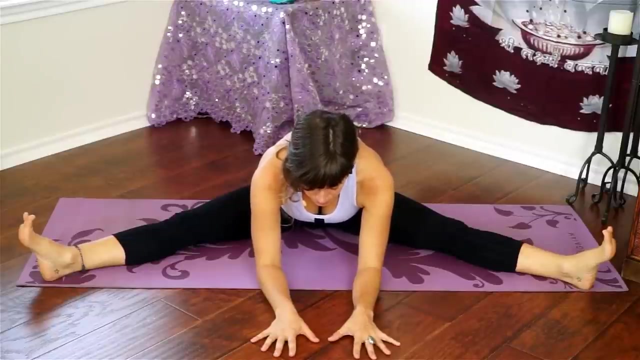 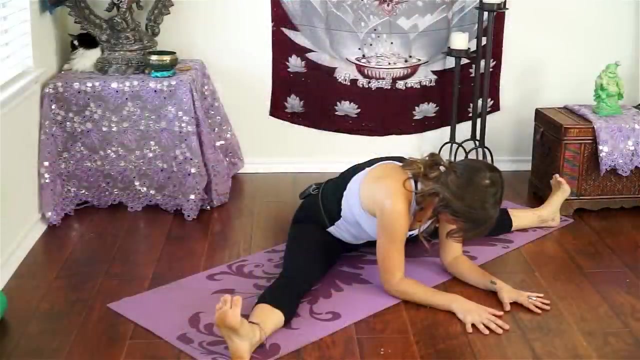 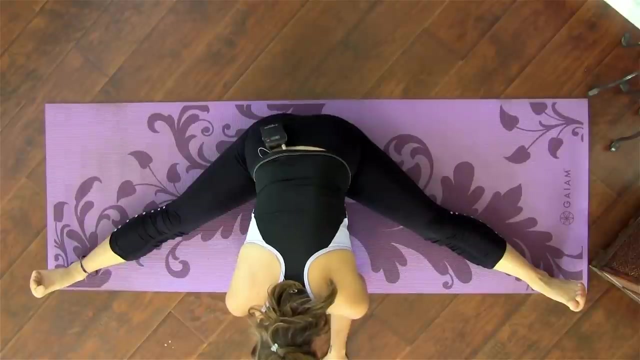 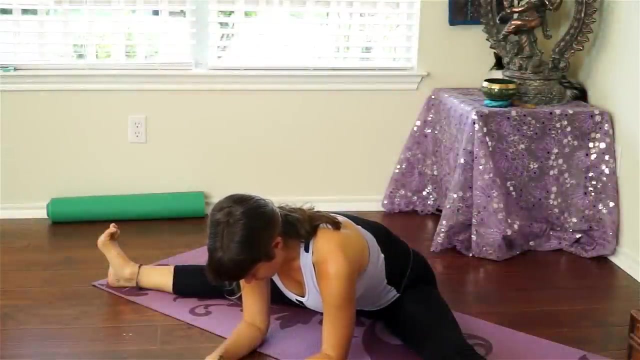 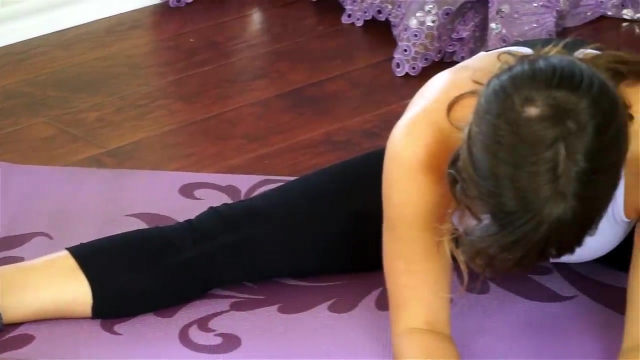 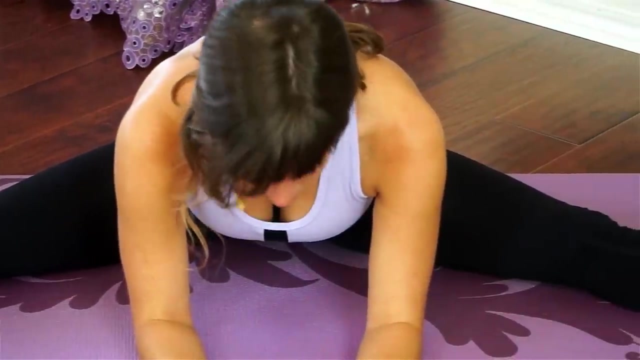 down the middle. you are welcome to explore this stretch in whatever way feels best for your body and always remember your slow and steady breath. 16: After a few minutes, your muscles are relaxed and comenzung to take care of their health. after 1-2 minutes you will feel. 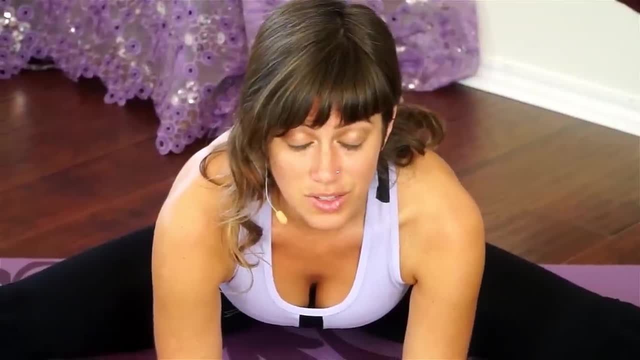 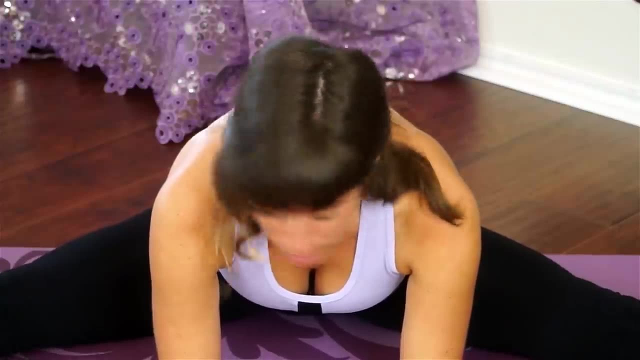 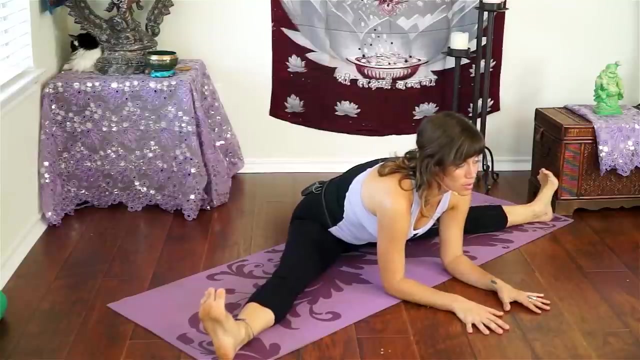 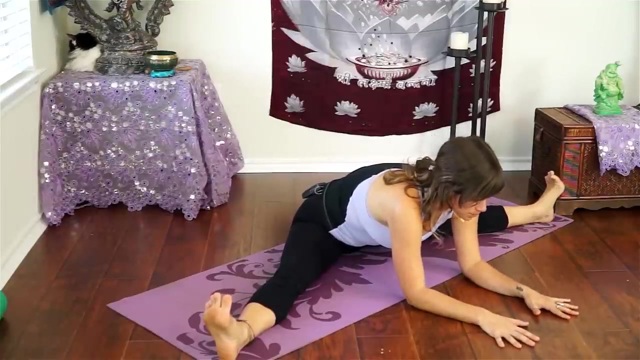 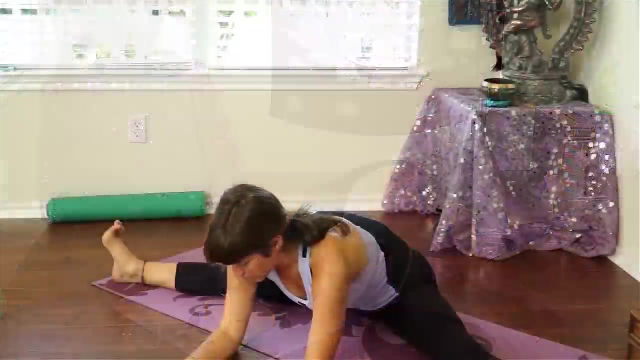 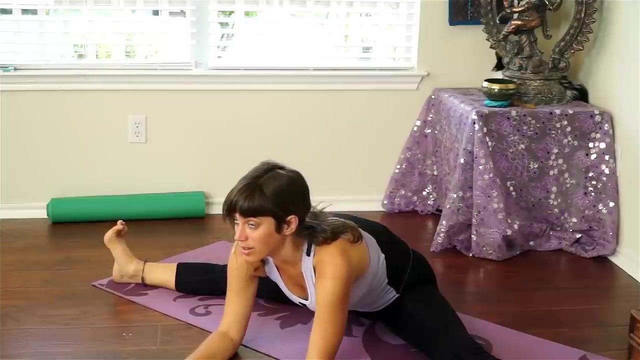 will start to relax. then you can start to take this a little bit deeper. you might open your feet a little wider apart, or you might find that you just want to come forward a little bit more, and I always find that whenever I'm having a hard time sleeping, if I take 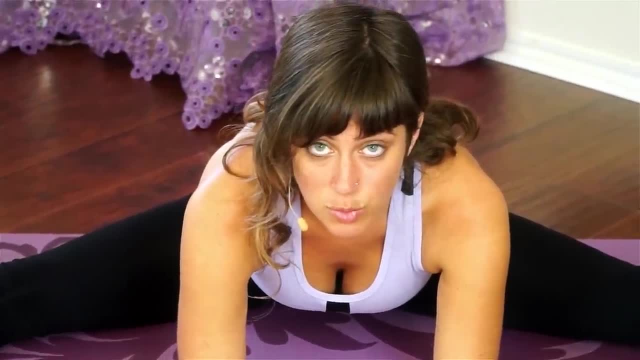 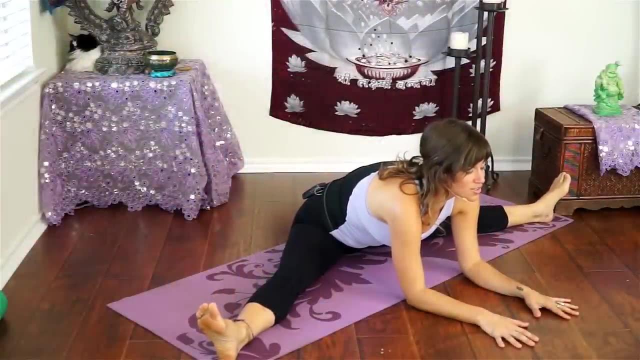 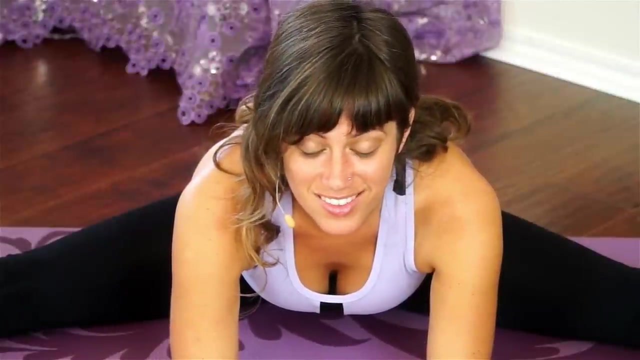 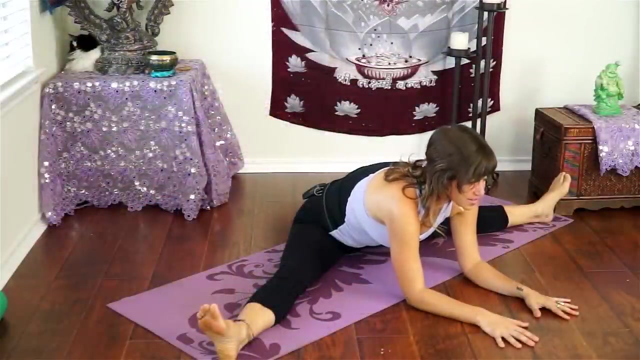 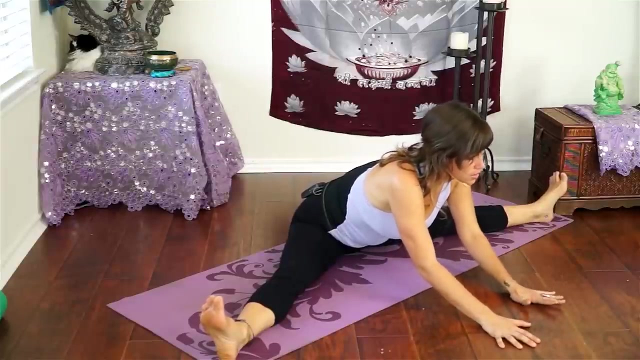 just a few minutes to do some of these basic stretches. it helps me to get out of my head and start to relax my body so that it's easier to fall asleep when I'm ready. yeah, yoga is really helpful for that. the same way we came in, we'll start to move out by gently walking your hands up. 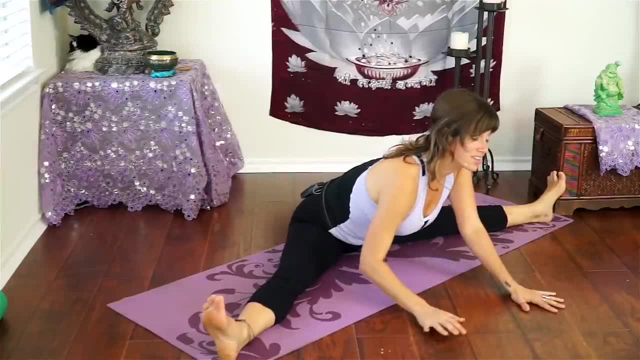 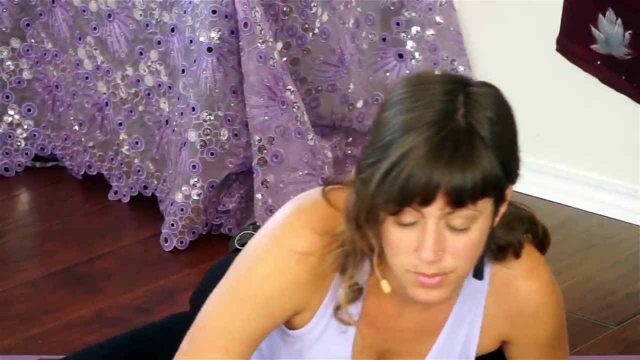 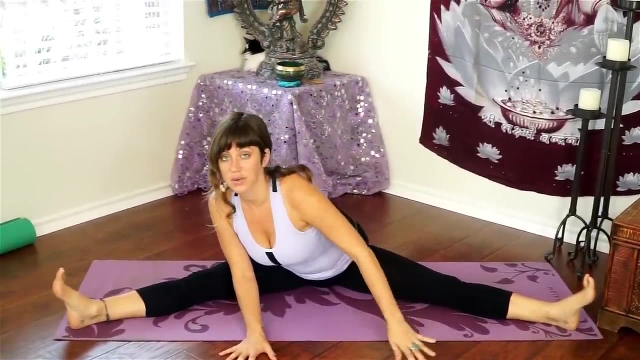 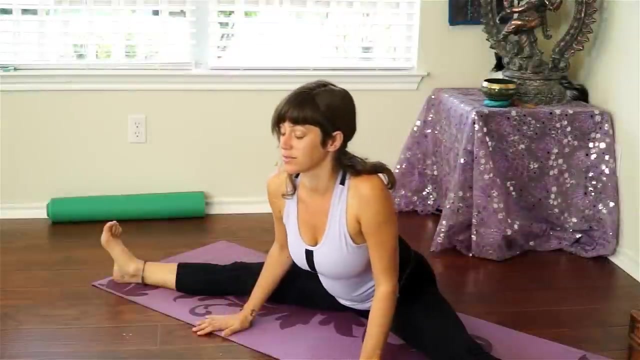 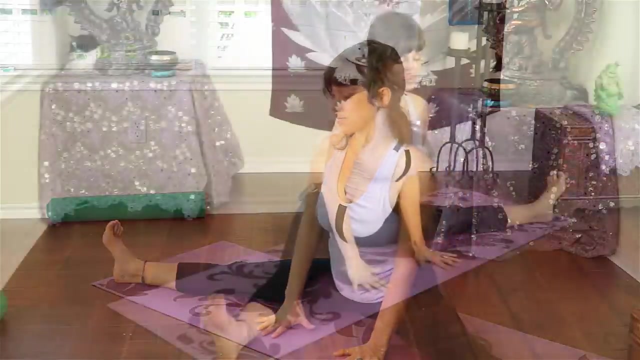 you can sway your body from side to side and bending your head for your hands, or forever just explore this movement in any way that feels good and supportive for your body. so much of our yoga practice is really about learning how to relax and stay absolutely comfortable back in your own cozy place next to your head, just for a 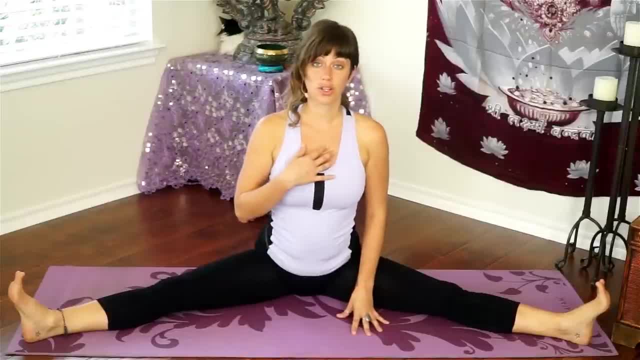 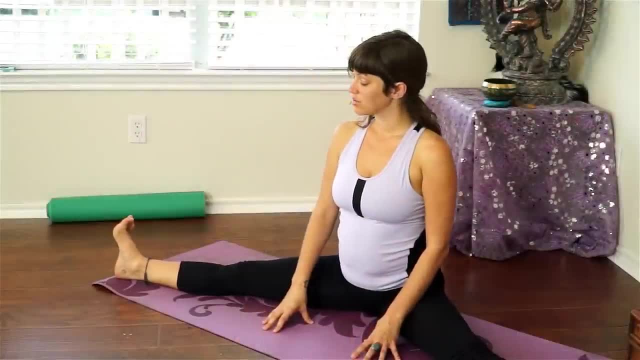 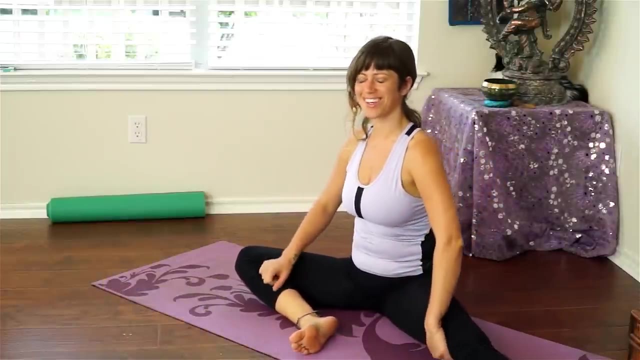 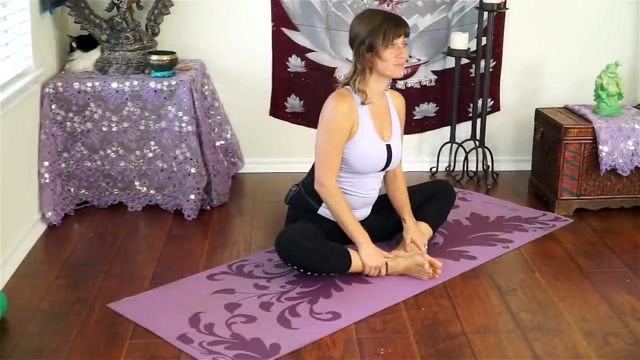 learning how to listen to your own inner voice and the wisdom of your own body. so go ahead and bend your knees. you can use your hands to help you so that you bring the soles of your feet together and again, if it's difficult for you to sit up straight here, 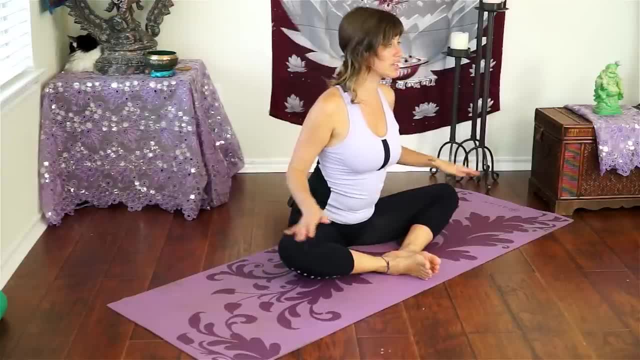 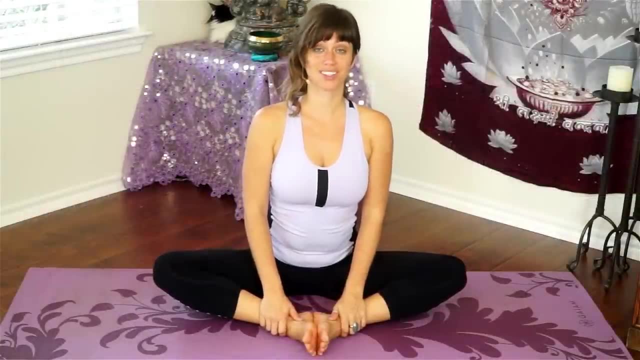 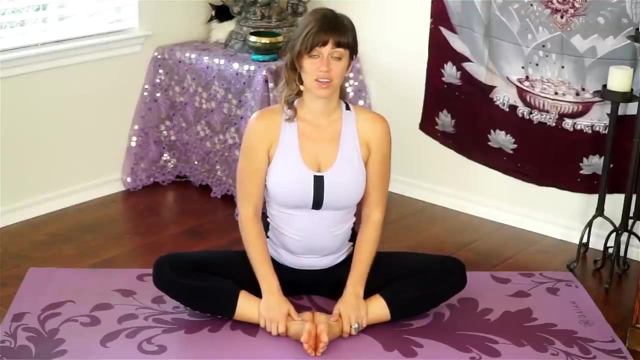 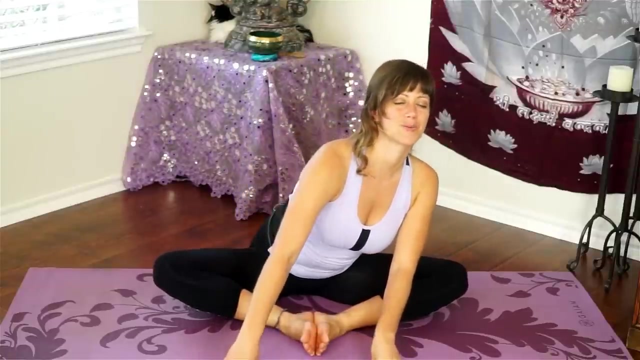 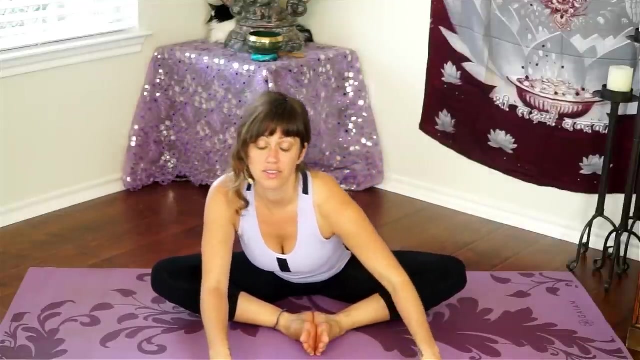 just sit on your pillow, sit on your blanket. anything that's gonna lift your hips a little higher will make it easier for you to sit up nice and tall and with your knees open out to the side. let's start to walk forward again and we'll just stick with the theme. here you can rock your body from side to side and just feel how. 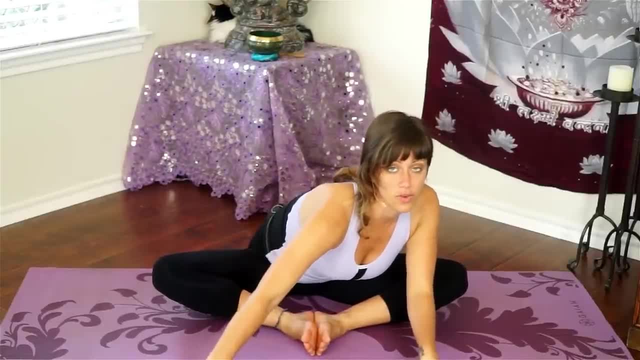 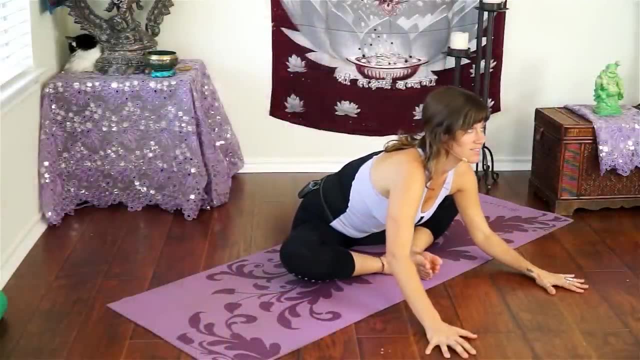 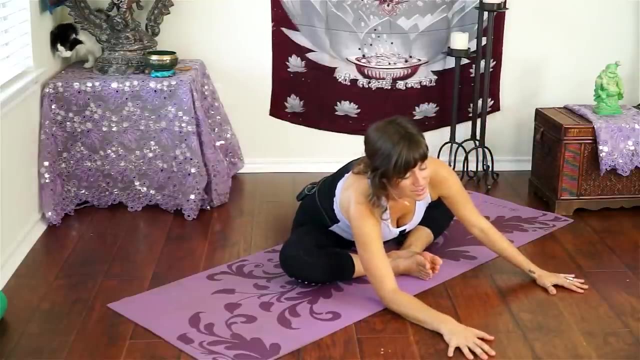 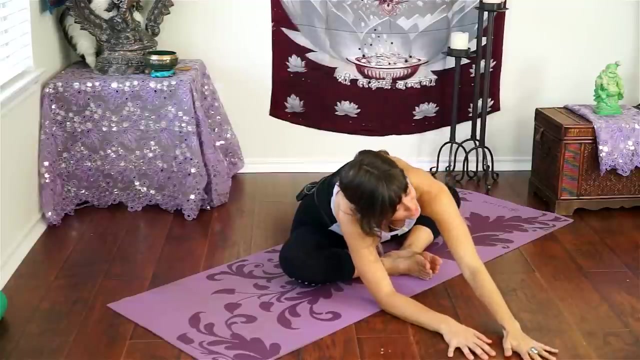 that stretch is different from right to left and you might find a spot that needs a little more love and you can stay there. so for me i'm feeling a little stretch on this left side here kind of feels good to just stay and stretch it a little longer. 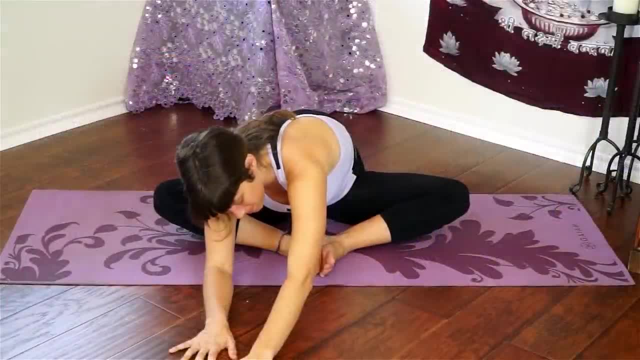 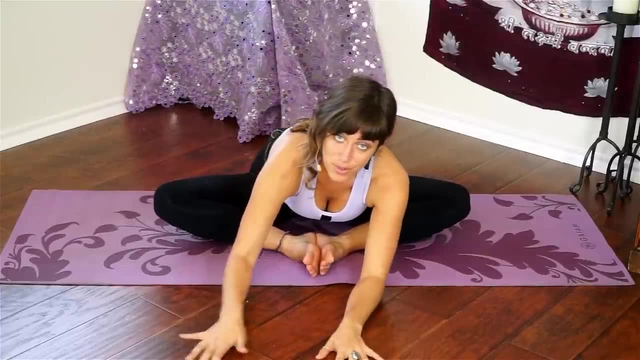 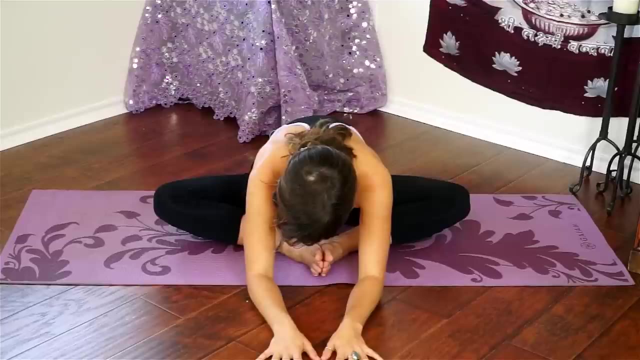 so you're welcome to honor your body in any way that feels the best for you. so, and when you're in the middle of the body and you're feeling a little stretch on your left side here, so for me, i'm feeling a little stretch on this left side here. 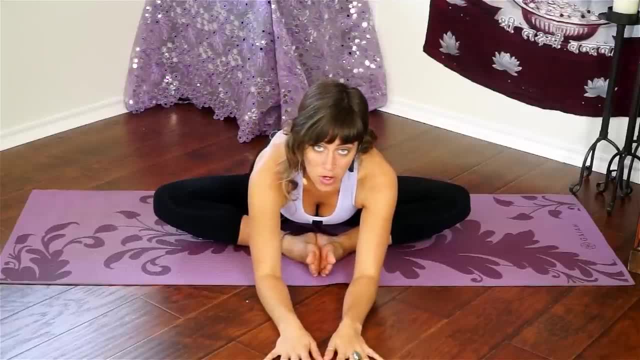 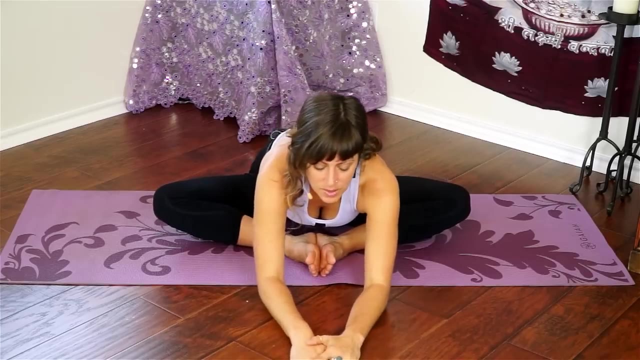 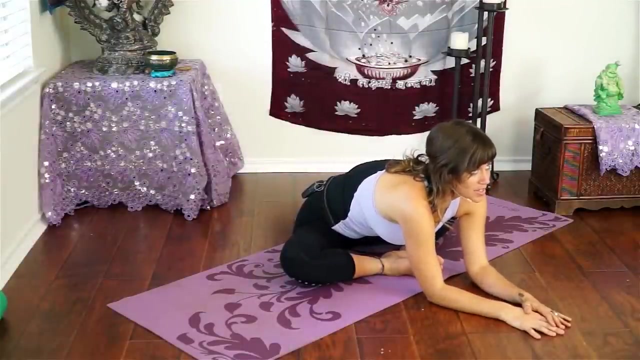 this stretch. it doesn't really matter how far you go, as long as you're getting that great stretching sensation wherever you need it the most. Sometimes people feel intimidated about doing yoga in a class because they're afraid that maybe other people will be watching or be judging, And that's one of the reasons that. 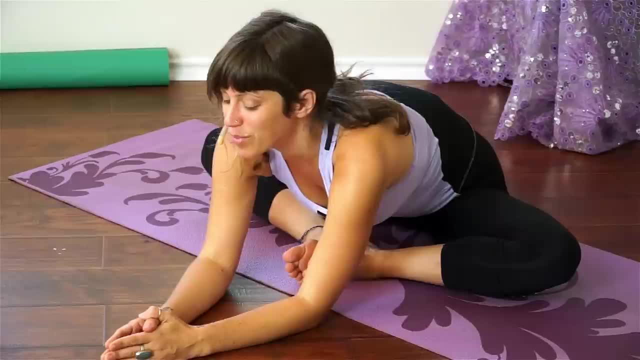 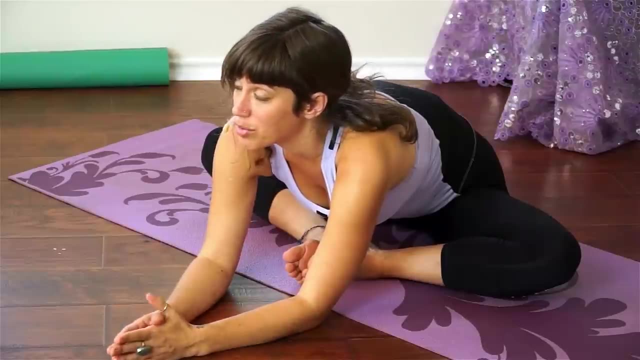 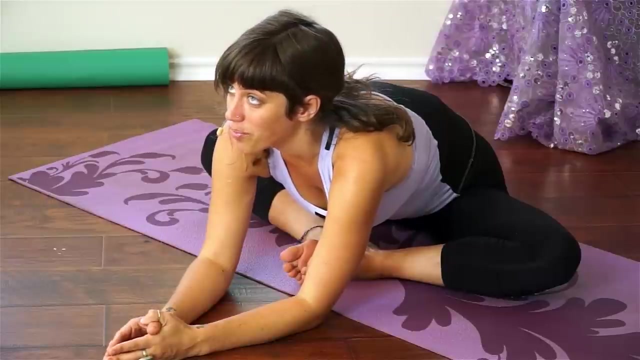 we wanted to make this series for you guys, this beginner's series, so that people like you that have never done yoga before or maybe a little nervous about it, can practice along with me in your own home and learn How important it is to always listen to the wisdom of your own body. so, even when 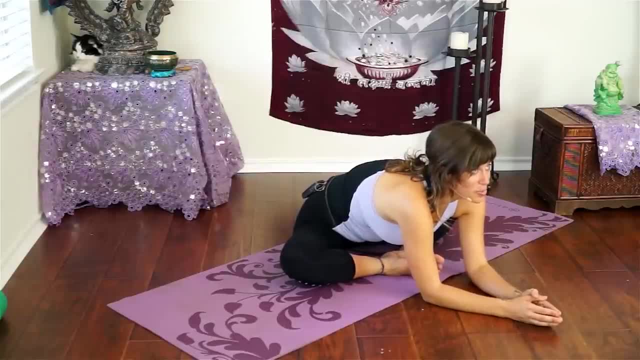 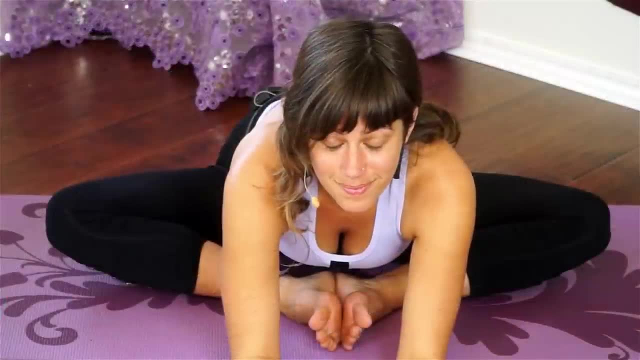 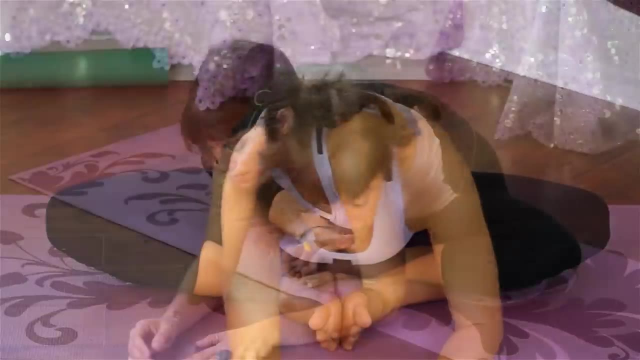 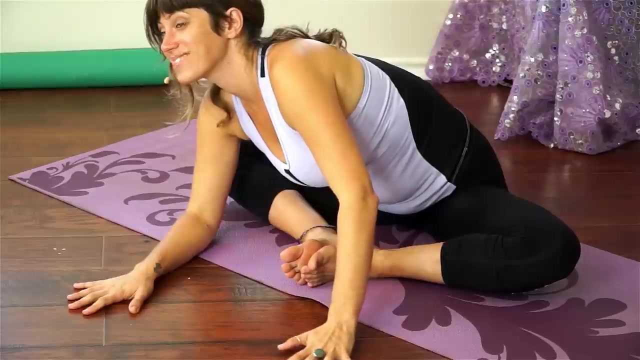 you go to a yoga class and there are other people around. it's always going to be your practice. Slowly start to come up, So I'm choosing to sway side to side. stretching my low back and my hips feels really nice. 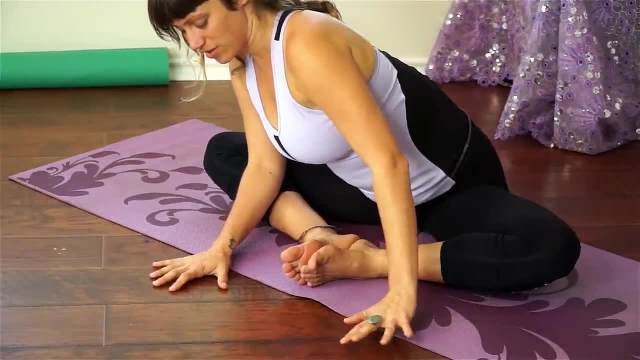 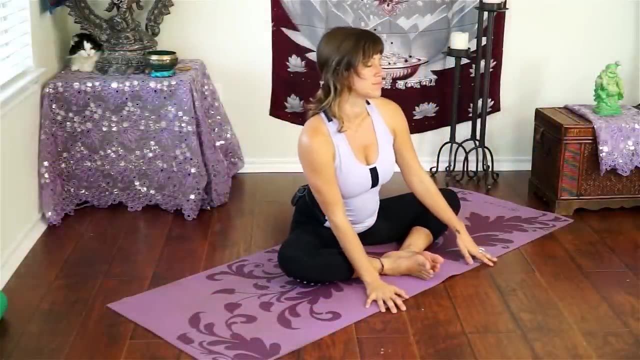 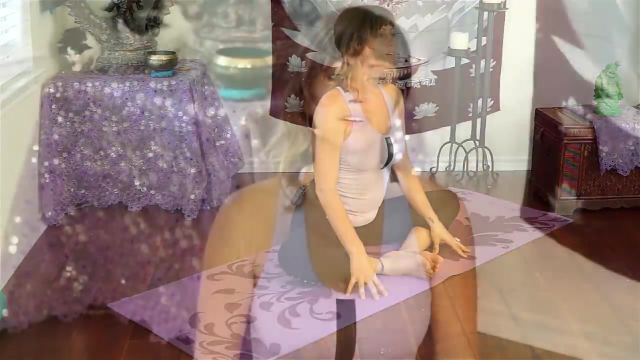 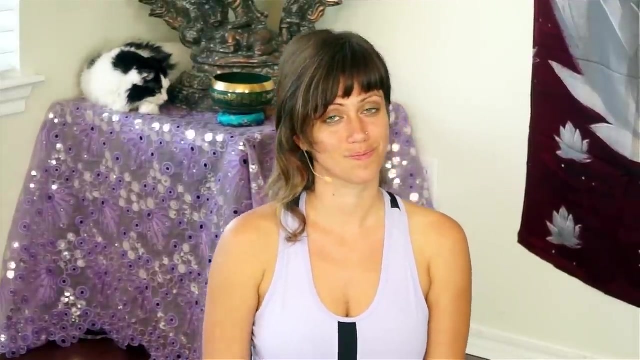 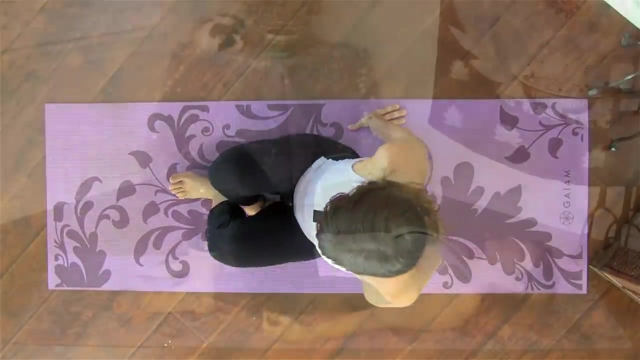 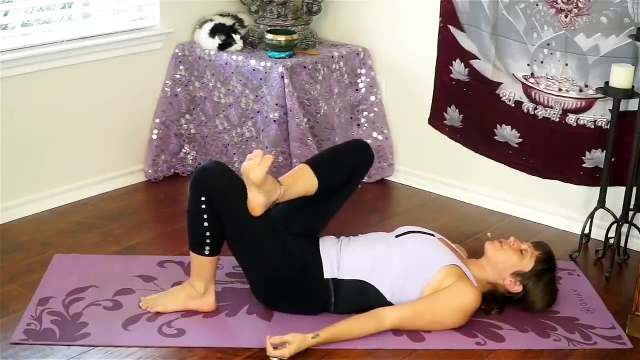 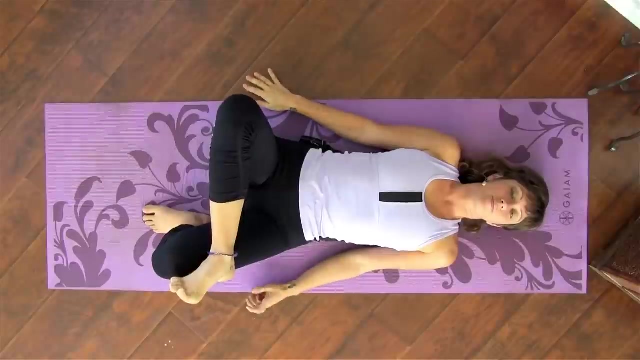 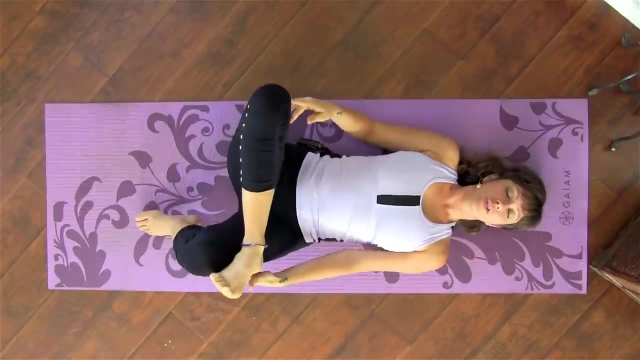 Slowly coming all the way up. Let's slowly start to make your way up, way onto your back lying down onto the floor. so once you're lying down, cross your right ankle over your left knee and open your right knee out to the side. keep this same shape in your legs and pull your left knee closer in towards. 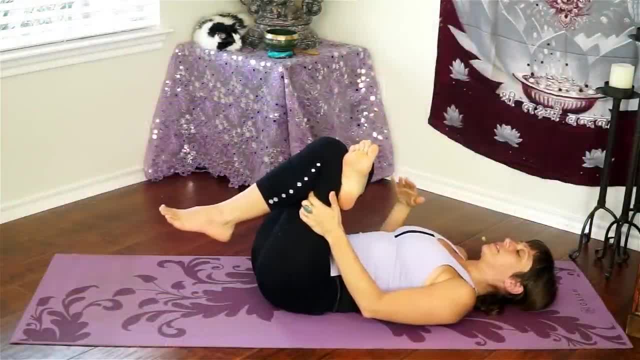 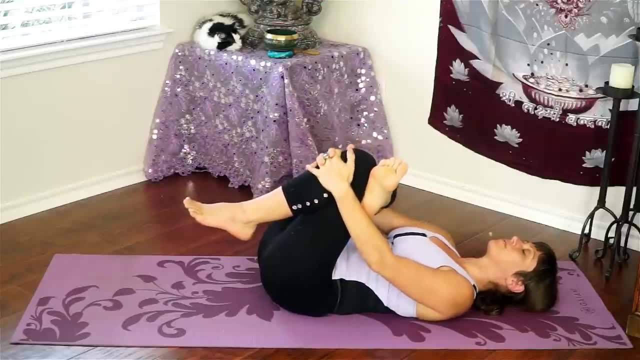 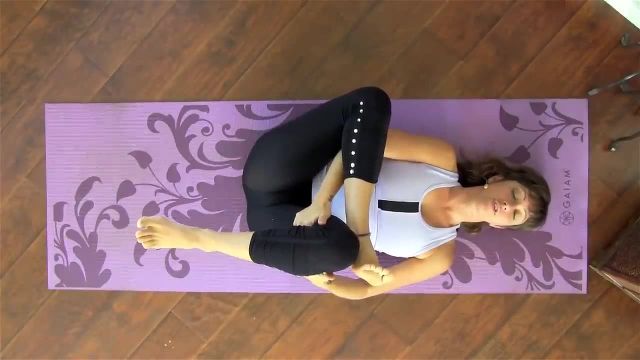 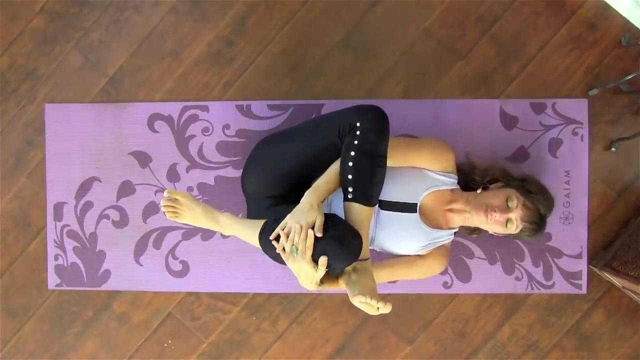 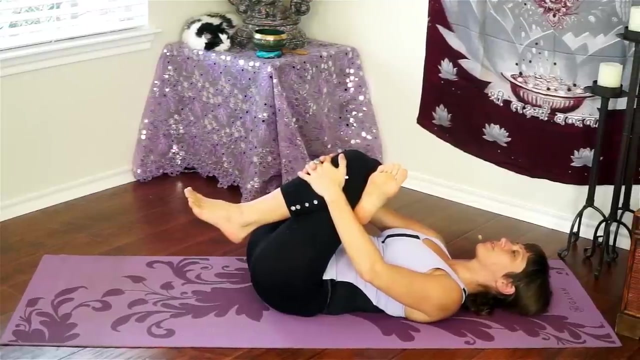 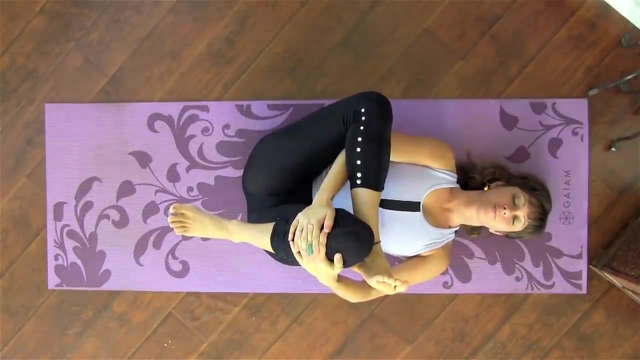 your chest. slide your right hand underneath your right leg to grab on to your left knee. you can also grab on to your left hamstring underneath your knee, if that feels better. either way is perfectly fine, and keep pressing your right knee away from you at the same time that you pull your left knee closer. you're going to feel a. 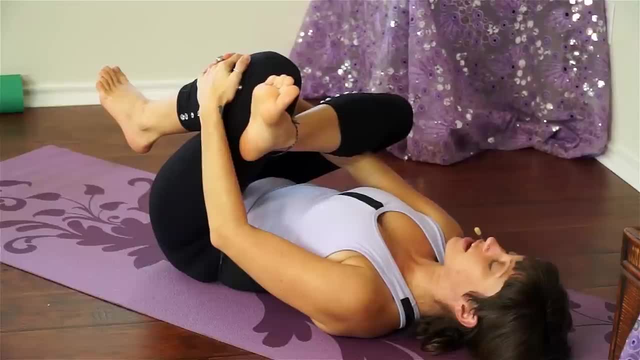 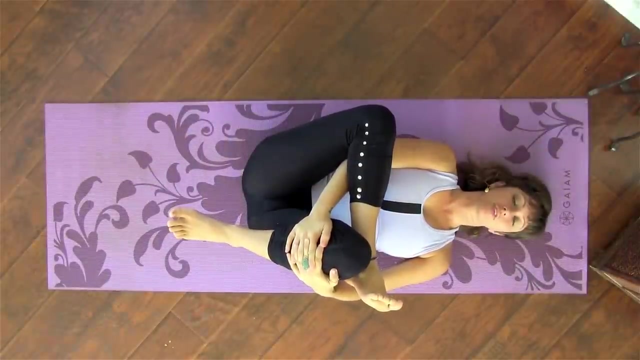 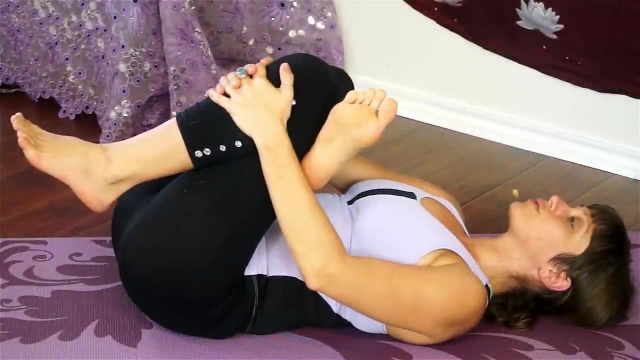 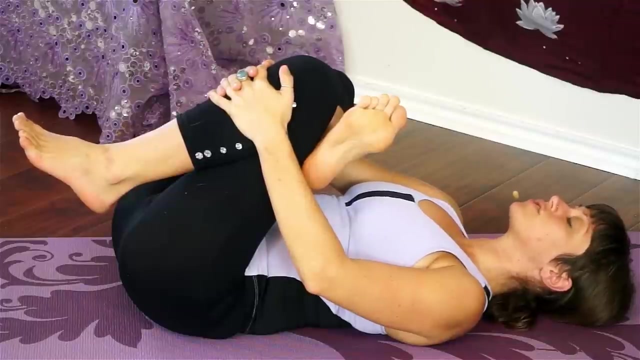 stretch across the outside of your right hip. this is an area that gets really tight for a lot of people, and the muscles here in your hips also contribute to sciatic pain. so if you're someone that deals with sciatica, this is a really effective stretch to release the tension. 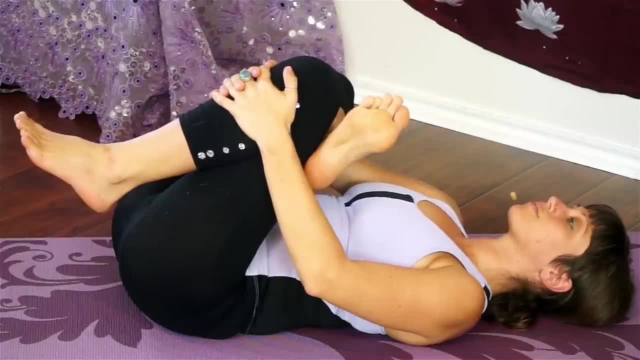 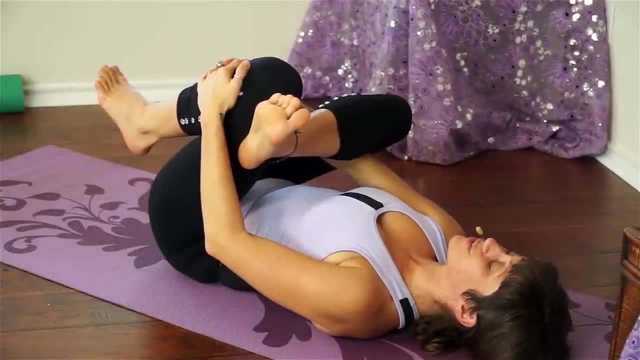 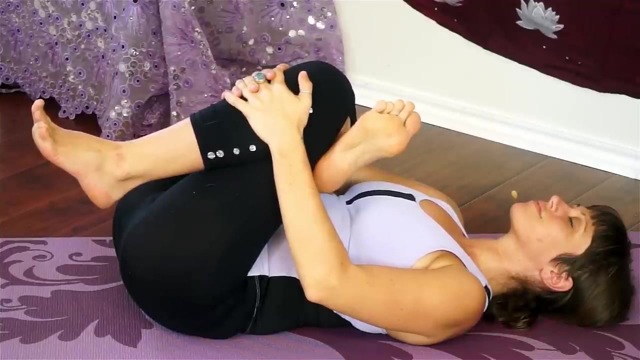 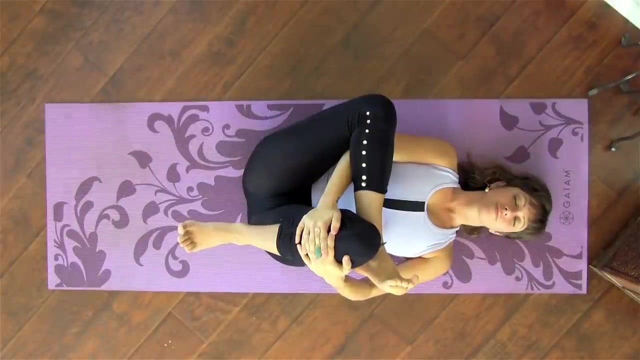 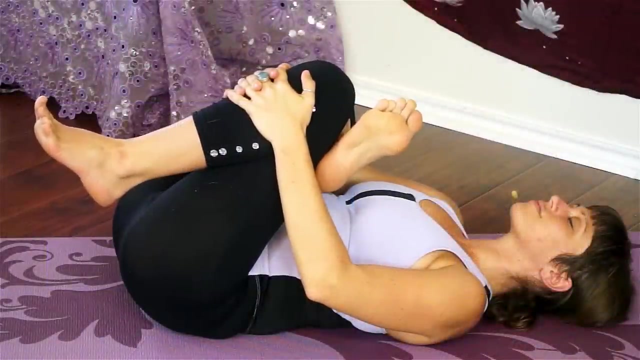 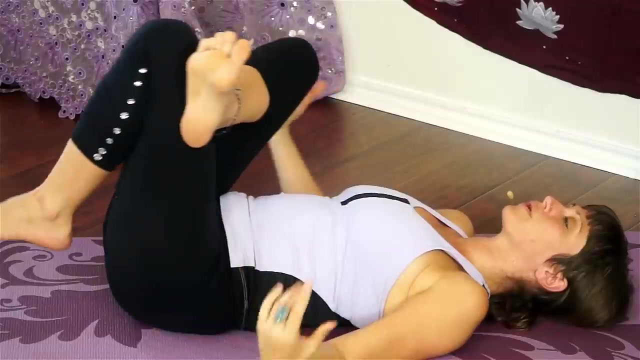 surrounding the sciatic nerve, so you can use this anytime, even if you're lying in bed. this is a nice, easy way to start to stretch into those glute muscles. you, you, you, you, you, you. you gently release your left leg and lower your foot back down to the floor and 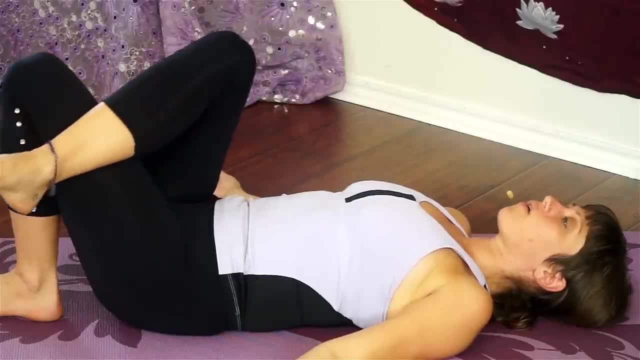 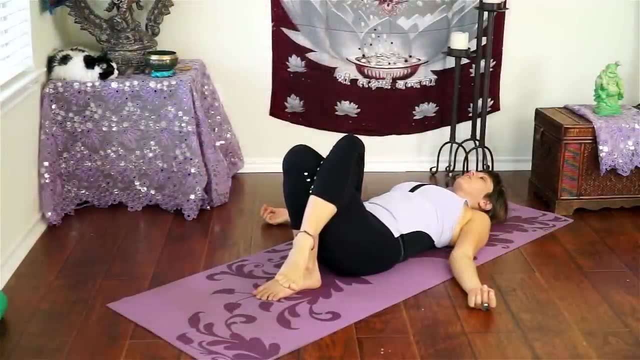 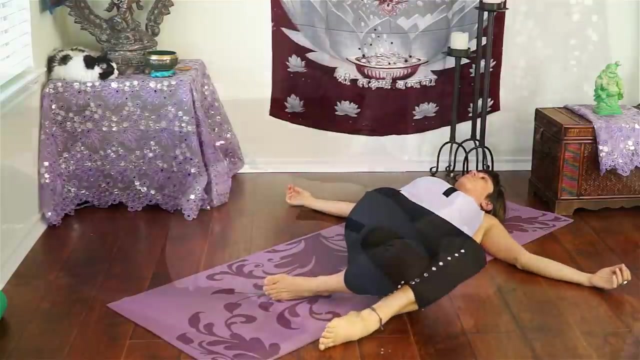 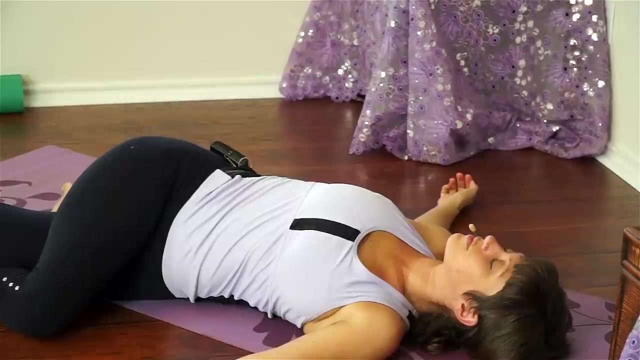 cross your right knee all the way over and then come back to the toilet seat, cross your right knee all the way over. now from here lower both knees over to the left, so this creates a nice twist in your spine. it helps to relieve tension across the low back. you can close your eyes here. 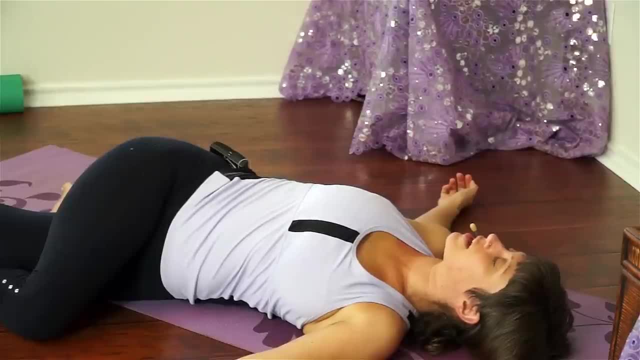 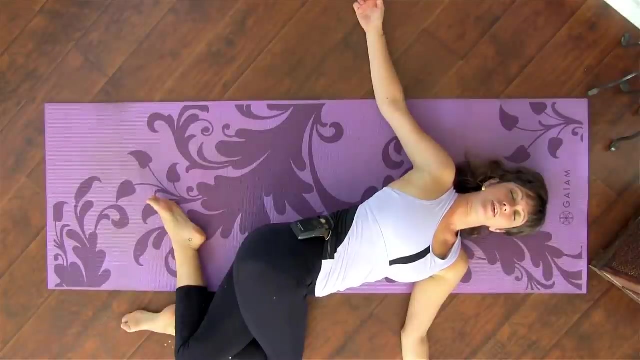 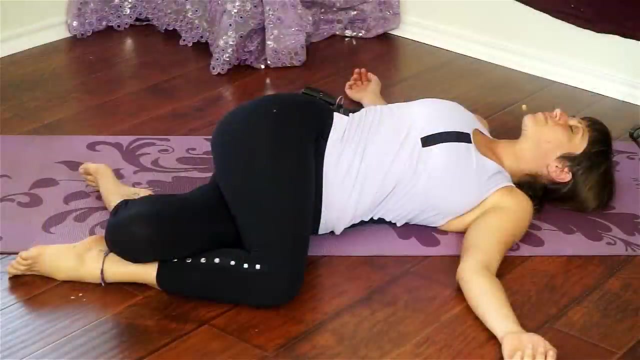 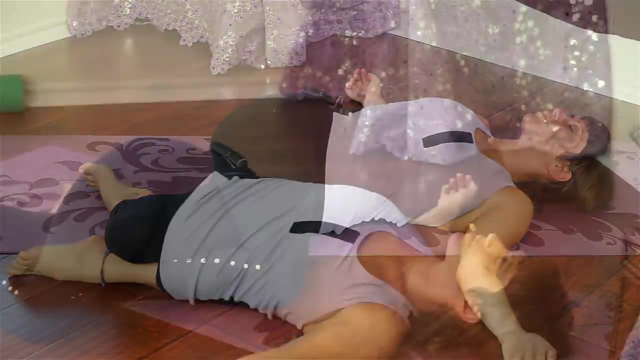 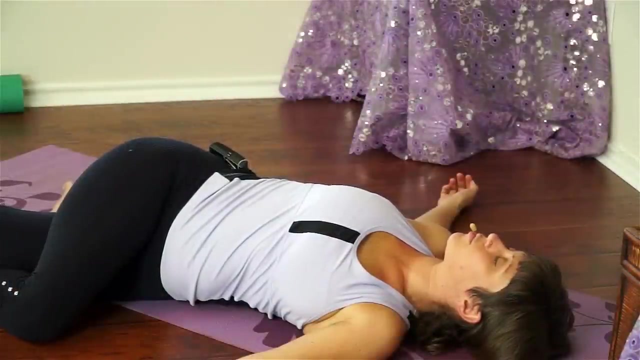 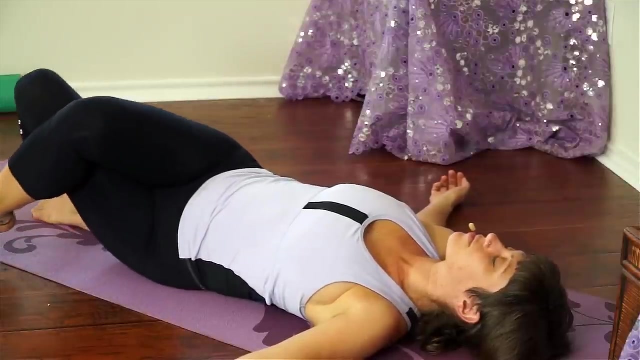 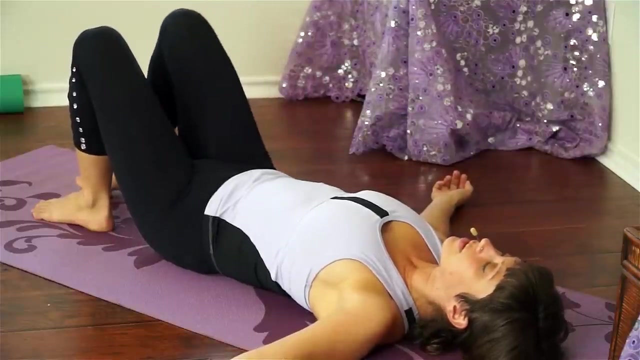 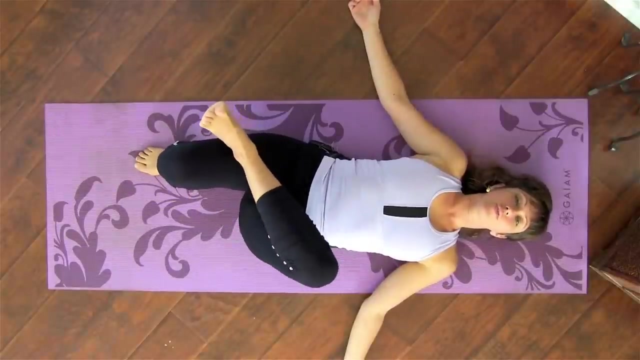 and let yourself relax. remember to stay connected to your slow and steady breath and then, as you're ready, we'll slowly start to come back to the center. nice and easy: uncross your right leg and then we'll switch to the other side. cross your left ankle over your right knee and open your left knee out to the 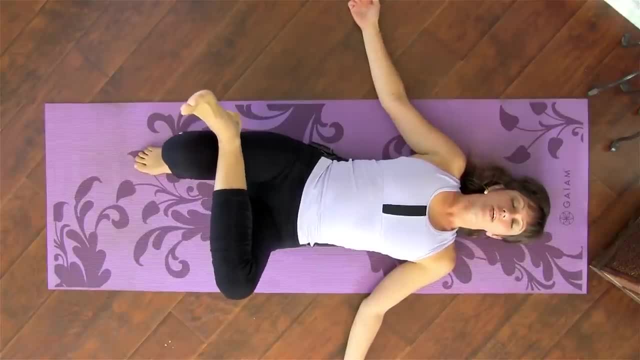 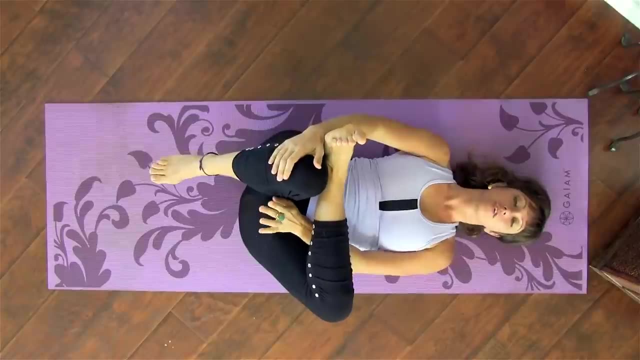 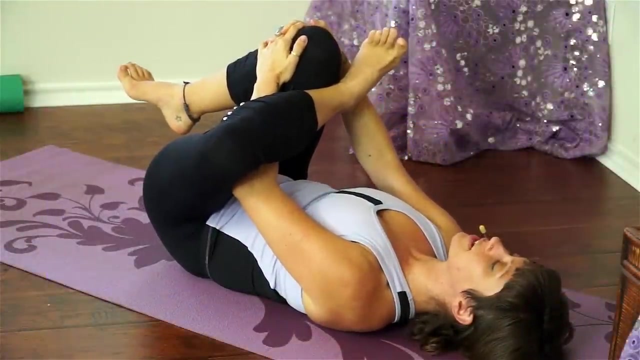 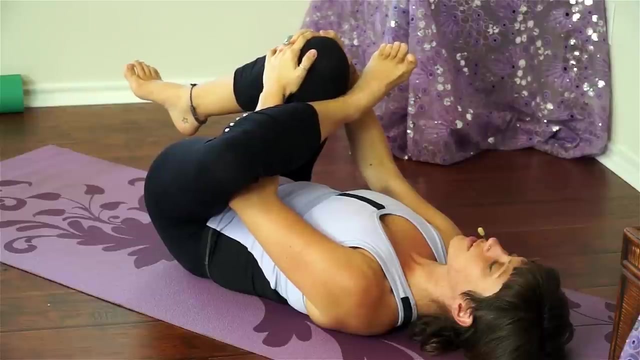 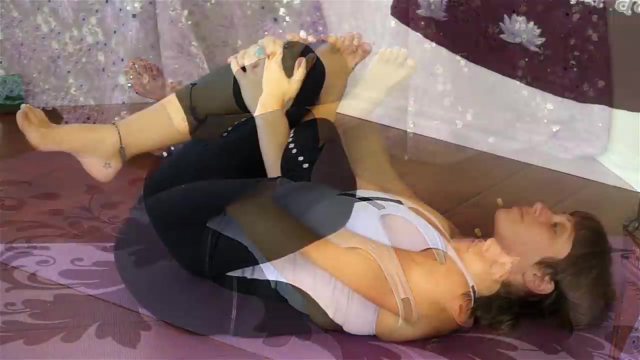 side, then draw your right knee and then draw your right knee and then draw your right knee towards your chest, lace your left arm underneath your left leg to grab onto your right knee and start to pull your knee closer to your chest at the same time that you press your left knee away. 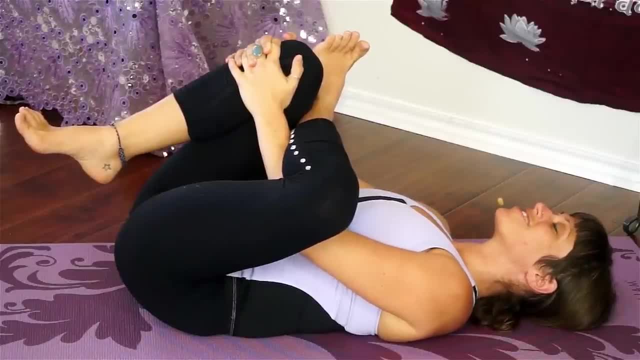 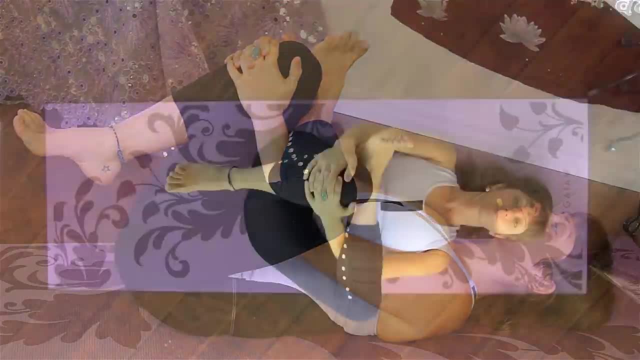 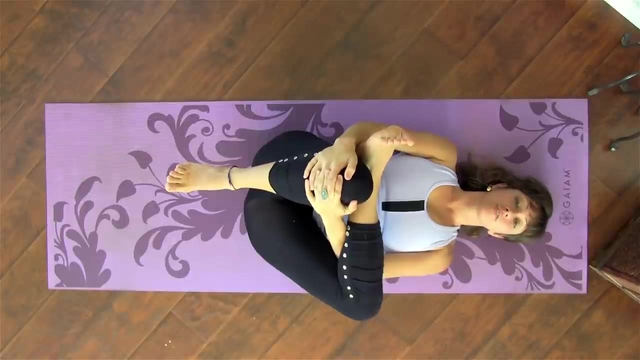 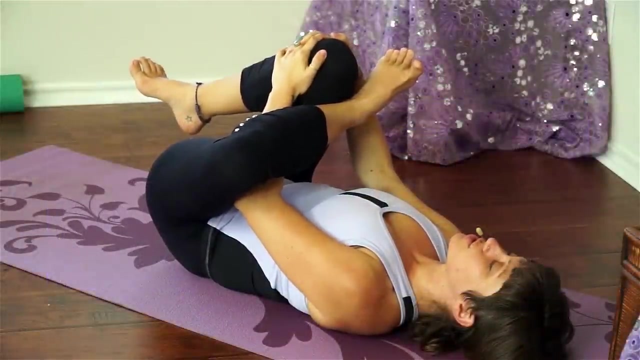 don't be surprised if you find that there's more tension on one side or the other. it's very common that we hold tension in an imbalanced way, so this is your chance simply to notice and observe your body as it moves forward and backward. whatever it is you're experiencing. 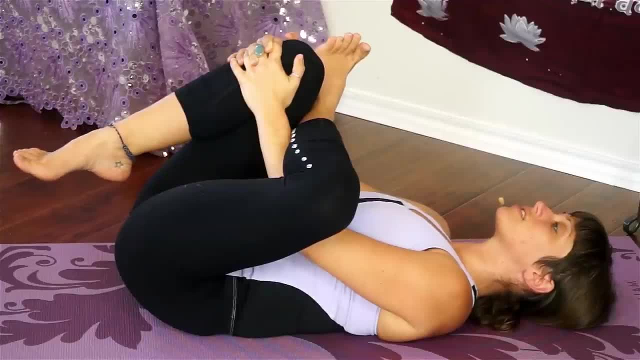 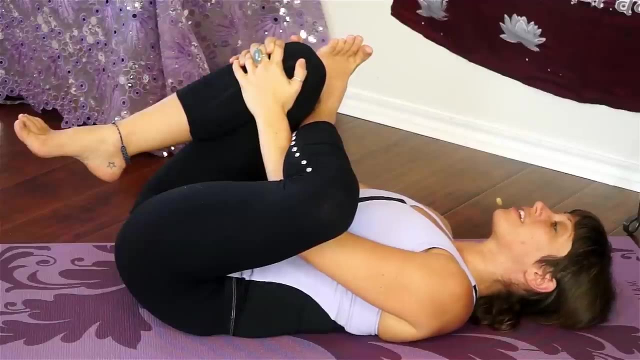 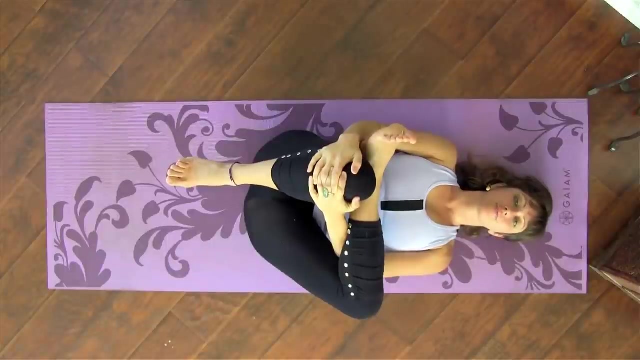 one of the important things yoga teaches us is how to witness our experience without judgment. so often in our lives, we are naturally judging situations as good as good and bad, when the reality is, it just is so. if this is something uncomfortable for you being in this stretch, 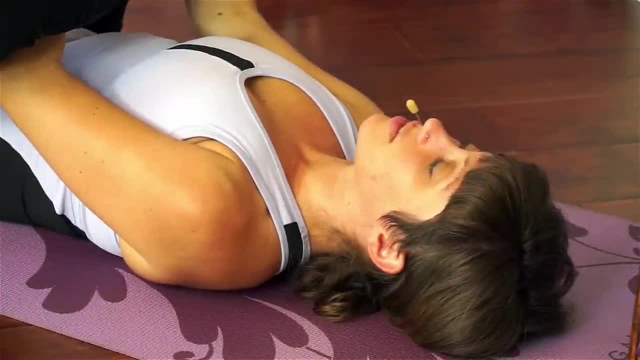 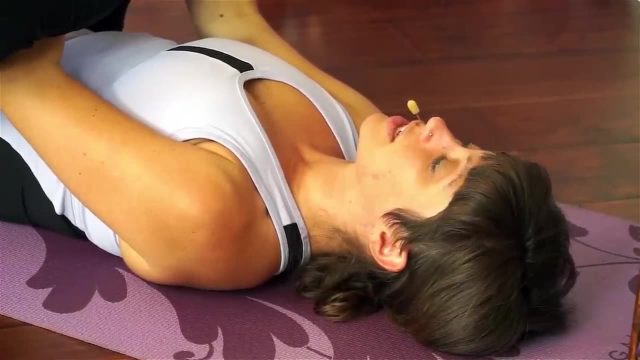 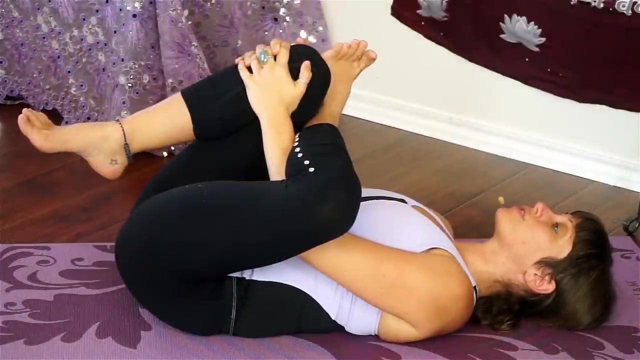 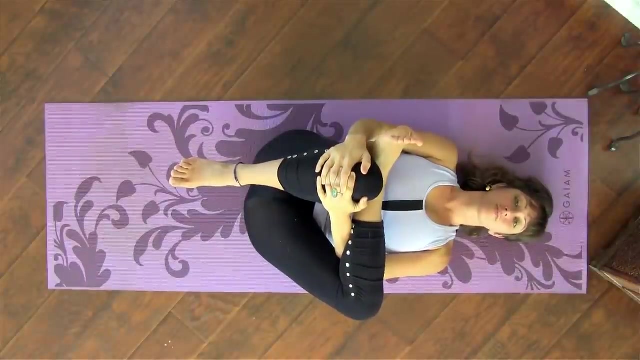 if the left side or the right side is more tense, the tendency might be to say: oh, this is my bad side, but there's really no need. neither side is good or bad, it just is. so witness your experience without making a judgment. simply see it for what it is. 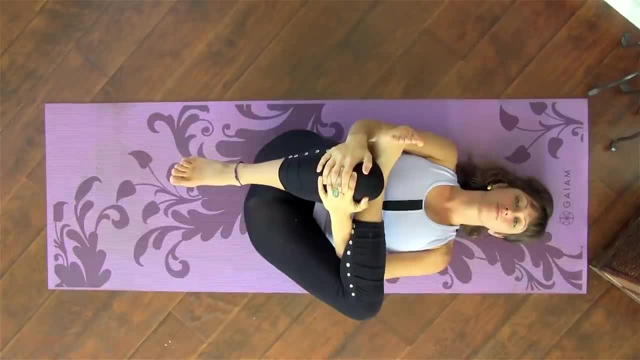 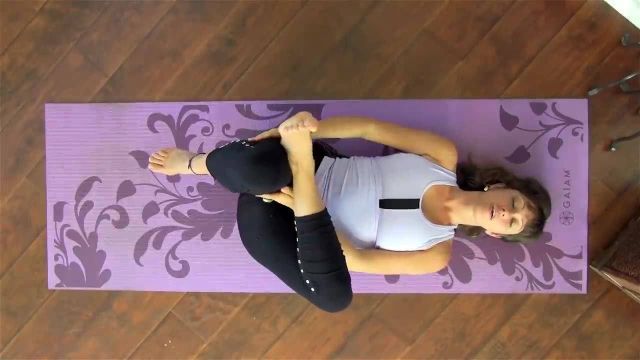 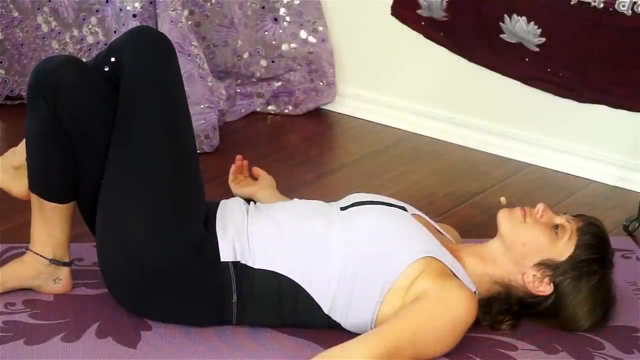 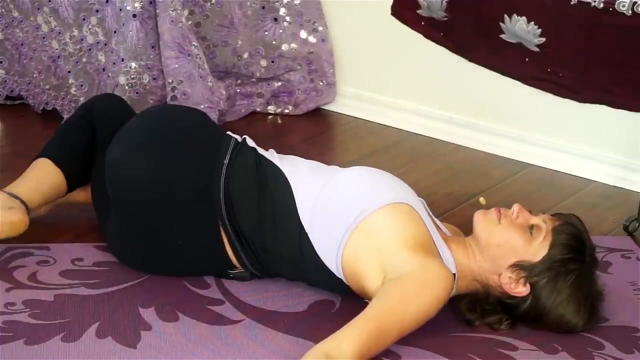 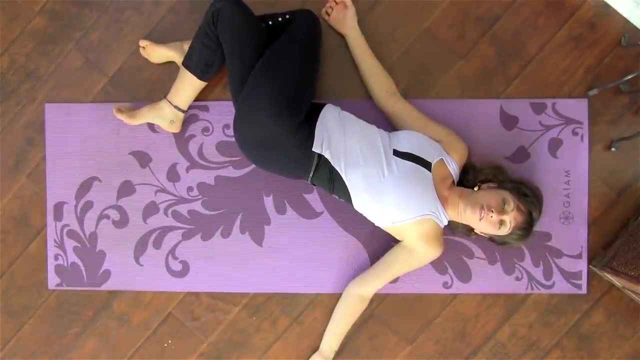 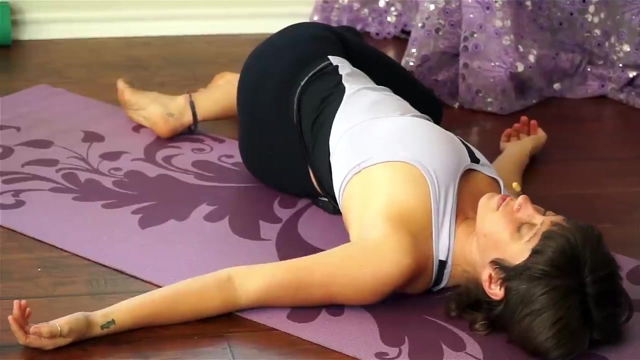 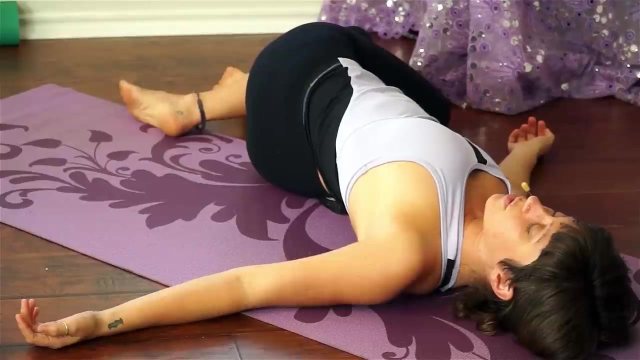 and release your right leg down and cross your left leg all the way over, then lower both knees to the right. now you have a twist on the other side and you have another opportunity to witness a new experience, so you can close your eyes and just observe. where might there be tension? 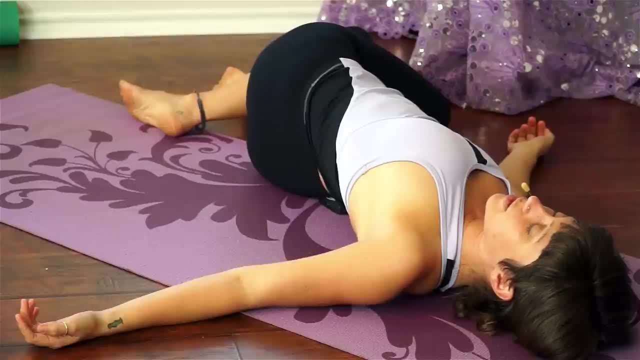 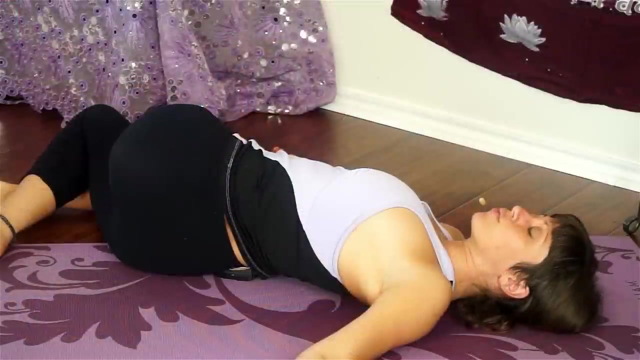 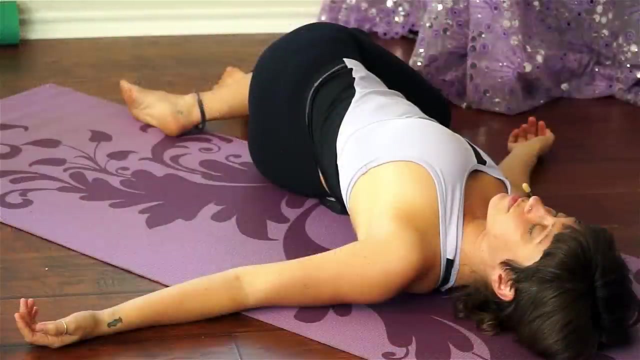 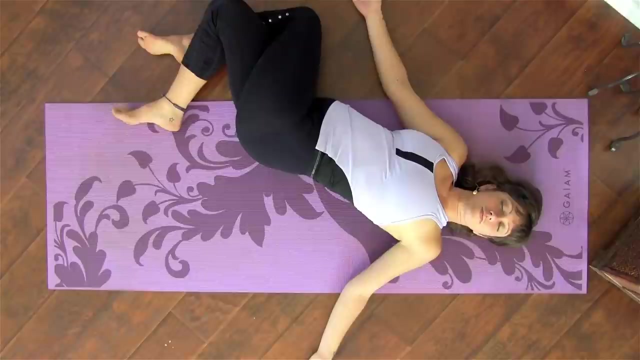 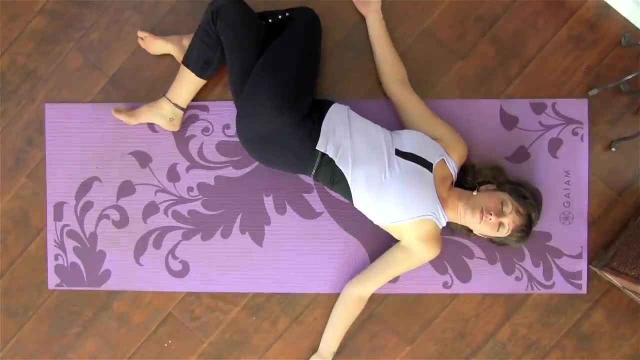 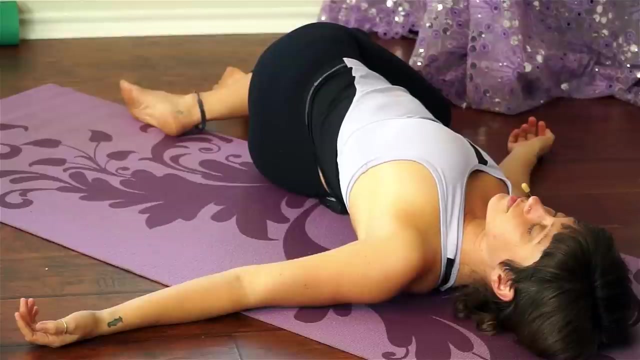 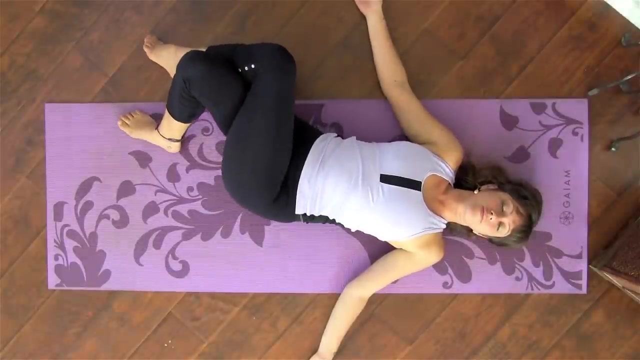 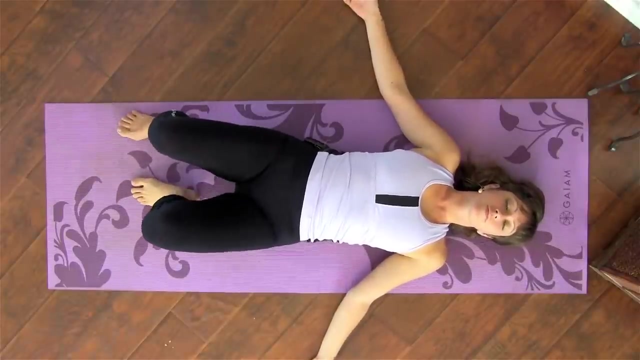 but it's also gonna go better. and the ¿you feel relaxed Chicken? huh, What am I doing? I got to go with my àquechette And then, as you're ready, slowly start to come back to center And uncross your left leg. 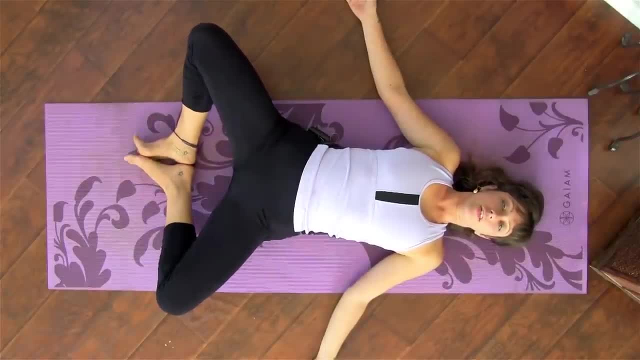 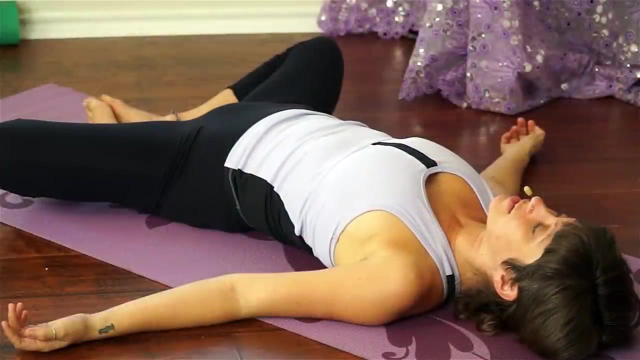 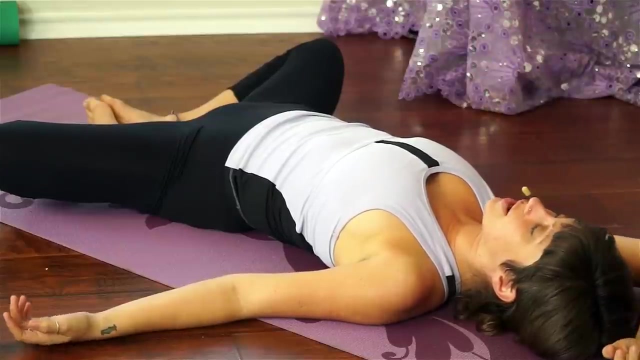 Then bring both feet together and let your knees fall out to the sides. And now gravity is going to do the work. Okay, Okay, Okay, And slowly, gently pull your knees open towards the sides. You can also bring your hands up overhead. 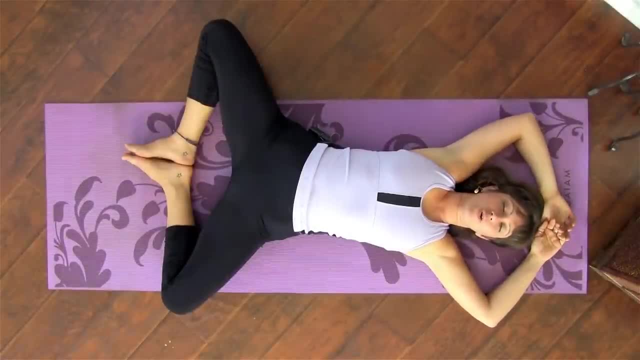 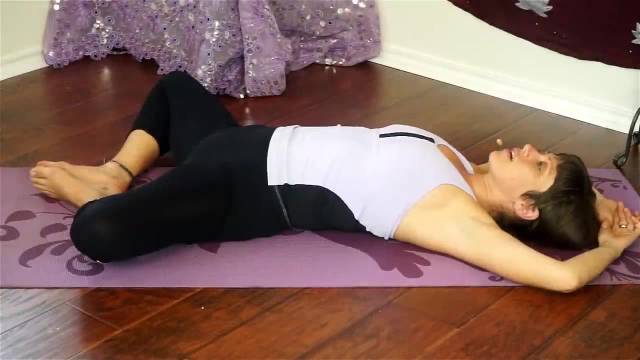 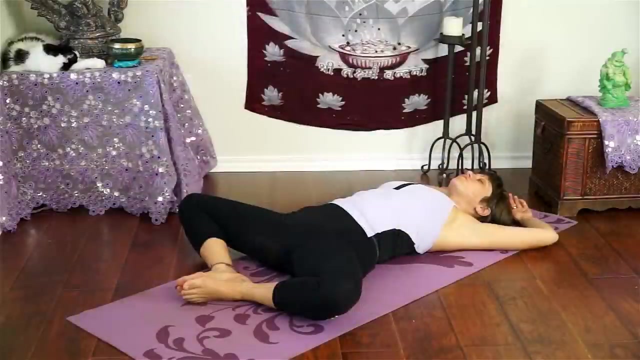 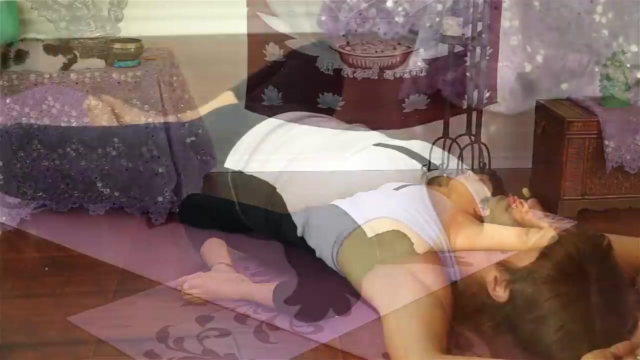 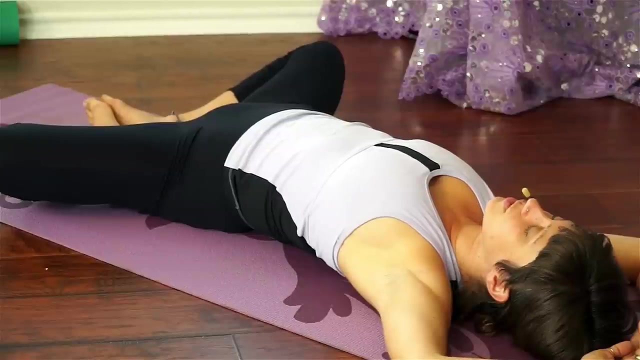 And this lets your armpits and chest be open, as well as your hips, And this is a very nice place to relax. You can also close your eyes here And just focus on your breath, Focus on the sensation in your hips. If your chest is very tight, you may also be experiencing a lot of sensation as your pecs start stretching. 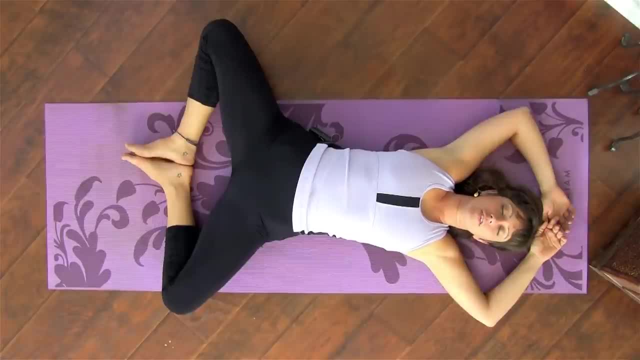 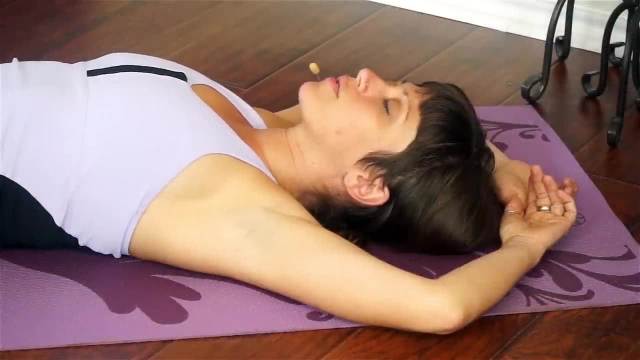 So don't let your thoughts be distracted. If your head is spinning around, you have to be careful and keep it in balance by all the other things we have to think about. But bring your thoughts right back here into your body. Watch your breath. 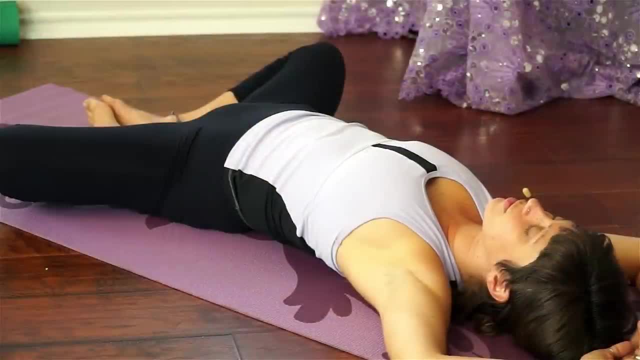 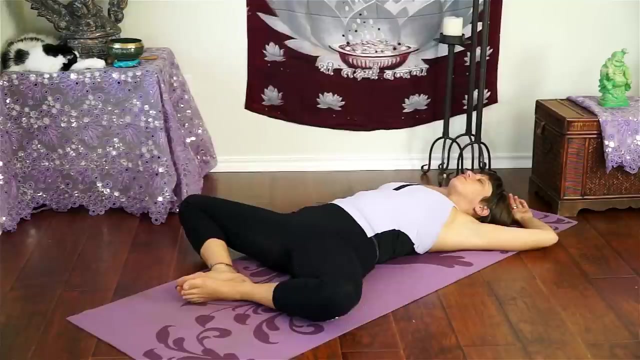 Feel it as it fills up your lungs And notice the change in your body. And, once again, the rest is very simple: Just make a new start and notice the change as it turns into an exhale and starts to escape your body. 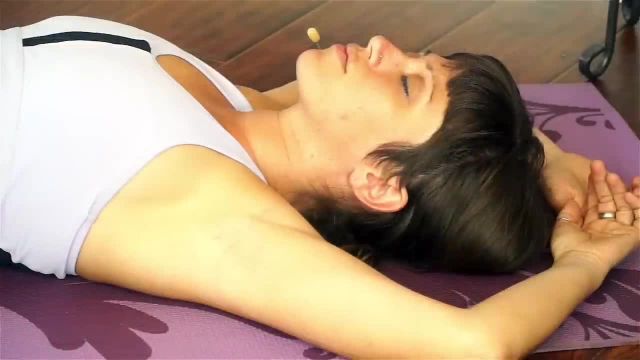 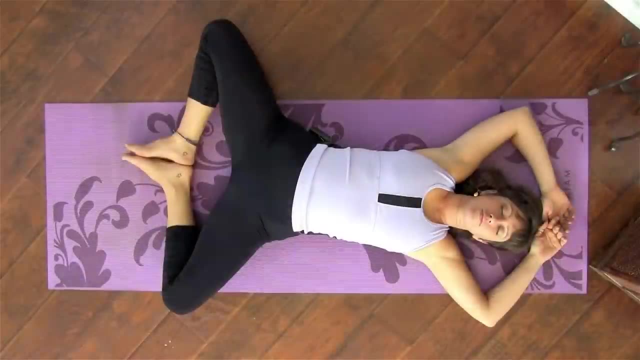 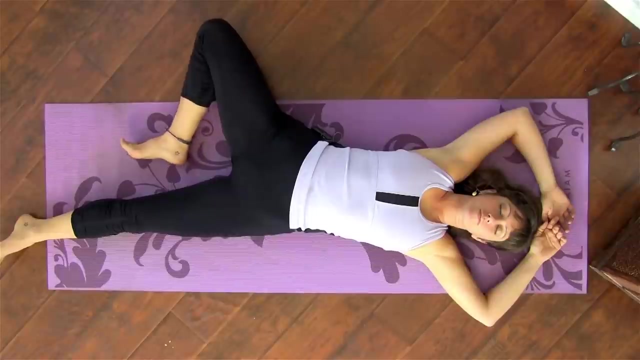 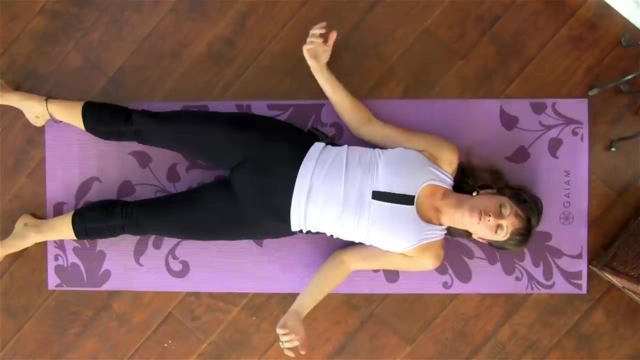 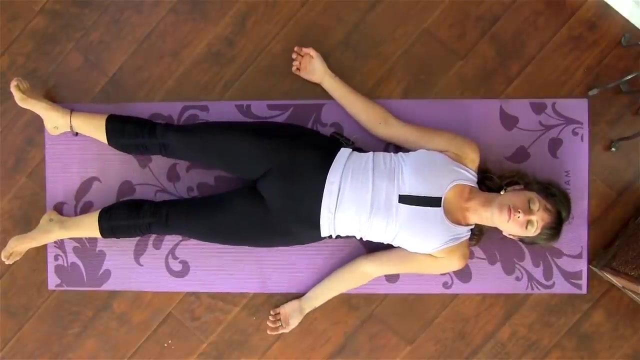 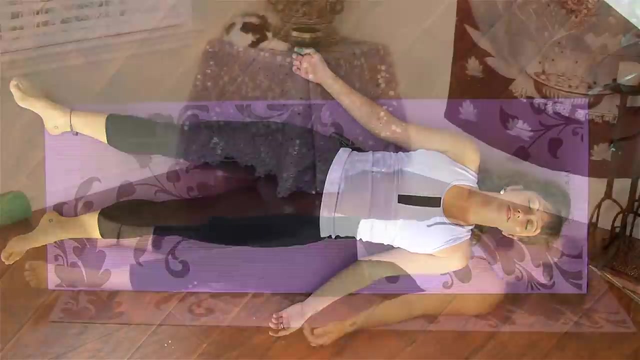 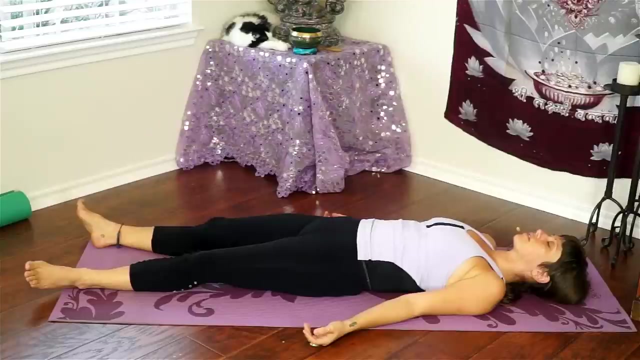 And then, whenever you are ready, you can slowly start to extend your legs all the way straight and let your arms go down, And then, whenever you are ready, you can slowly start to extend your legs all the way straight. And then, whenever you are ready, you can slowly start to extend your legs all the way straight. 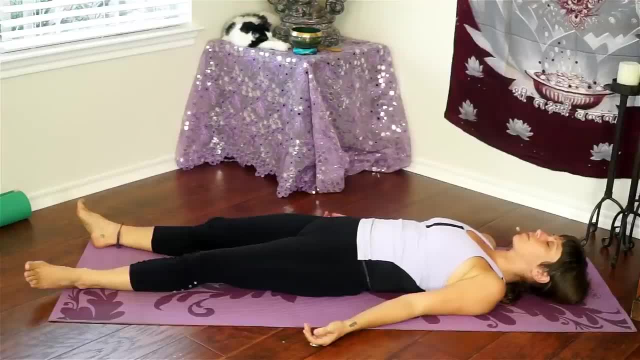 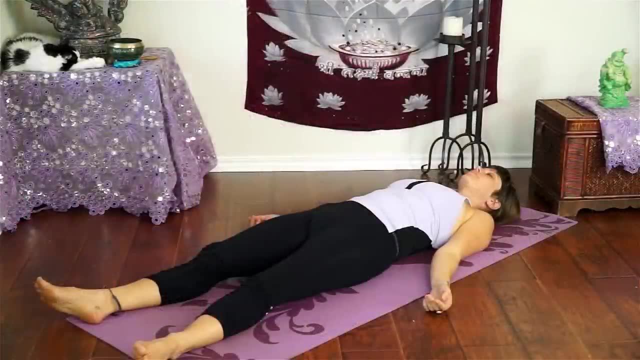 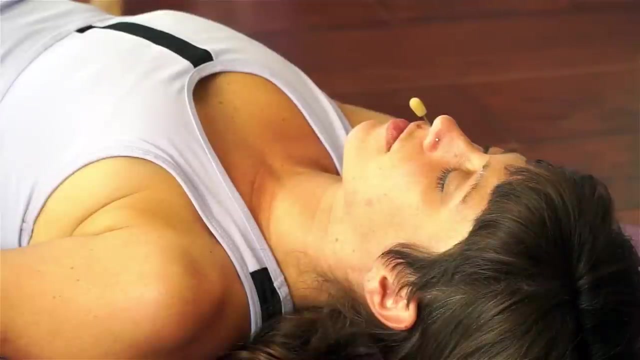 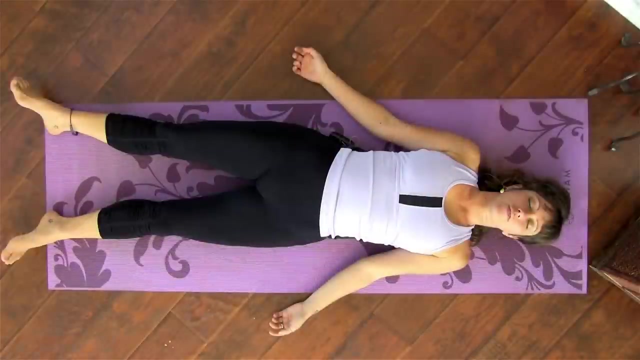 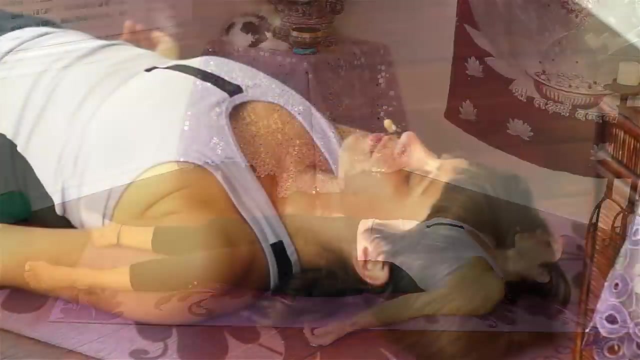 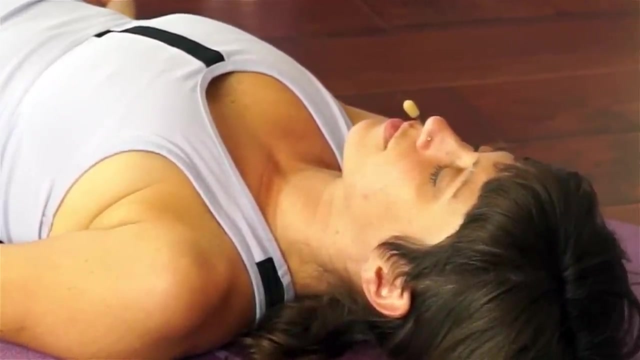 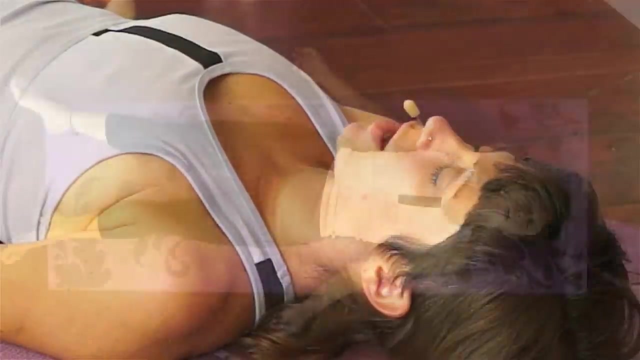 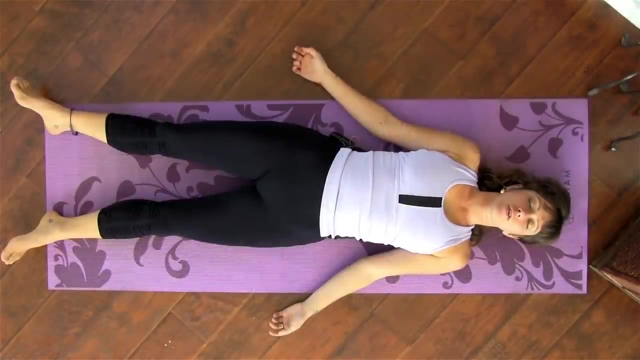 Let your tongue fall down into your mouth, away from your teeth, Stay connected to the rhythm of your breath And feel the residual sensations from taking this time to stretch your body. You are welcome to enjoy this moment of rest for as long as you need. 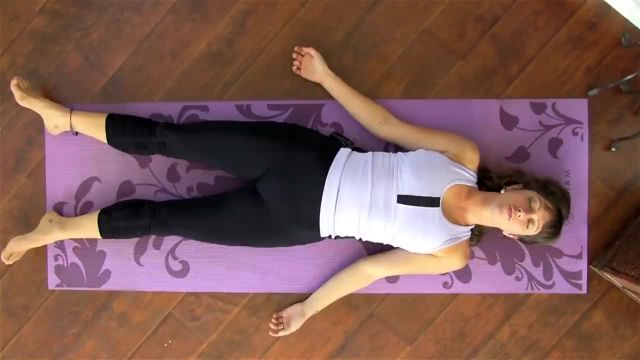 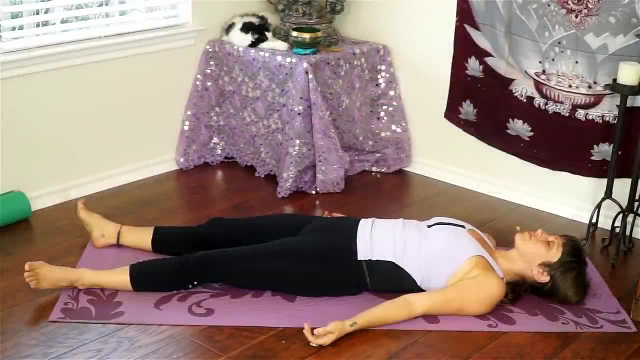 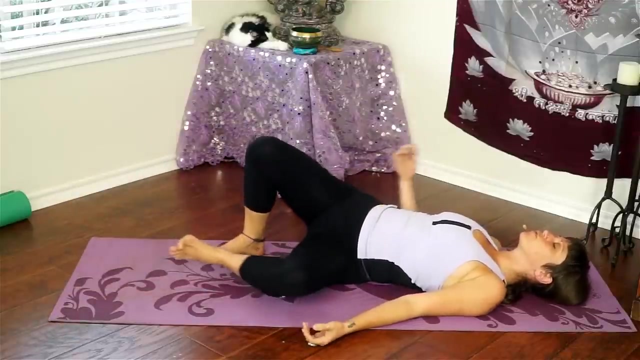 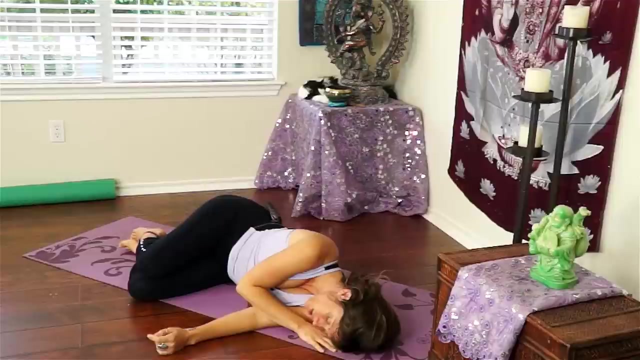 Some of you may even want to drift off to sleep. Okay, Good, And when you feel complete with your practice, slowly roll over to one side. See if you can keep your eyes closed as you move, And just gently laying onto one side. 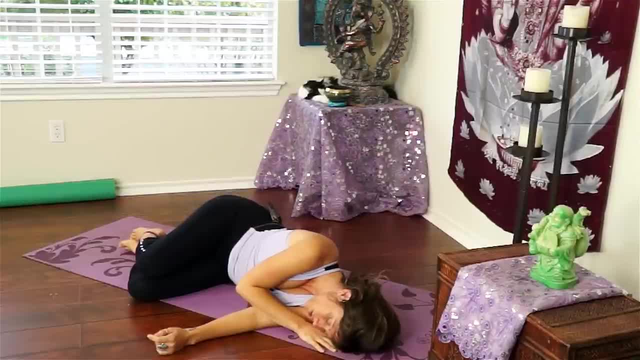 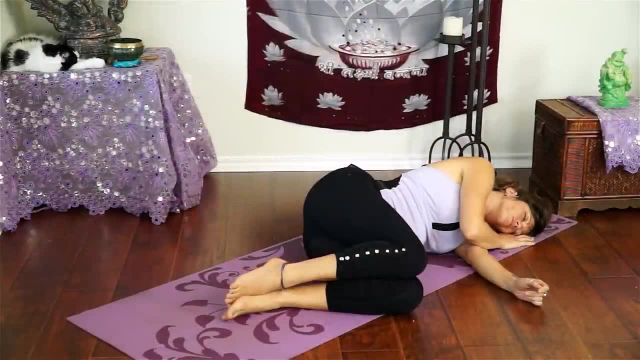 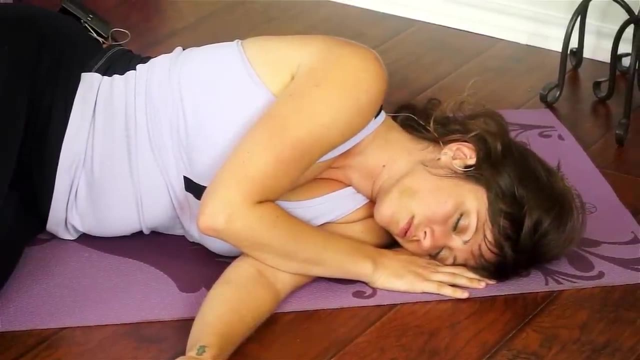 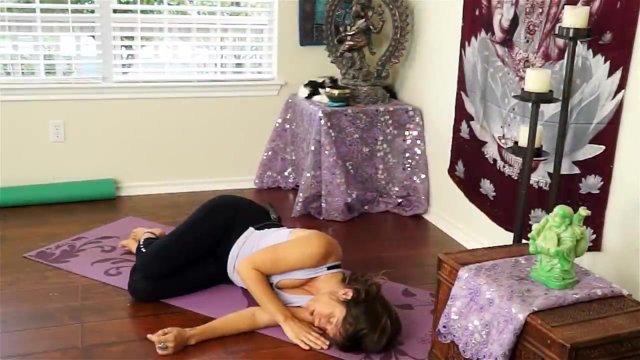 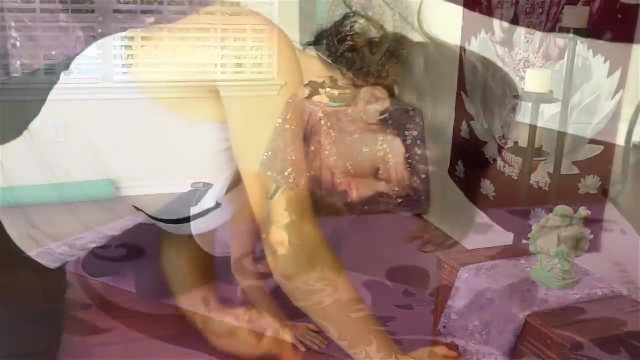 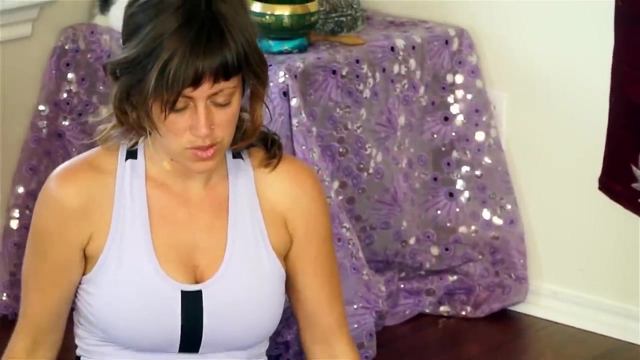 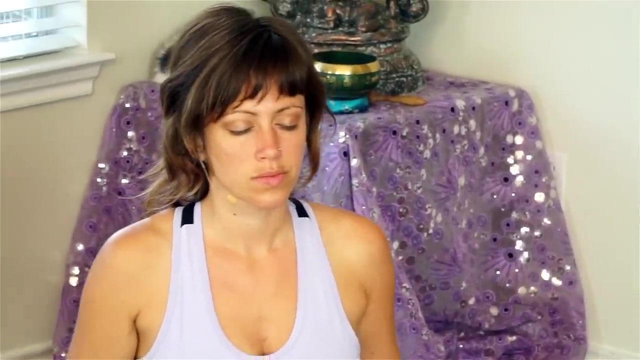 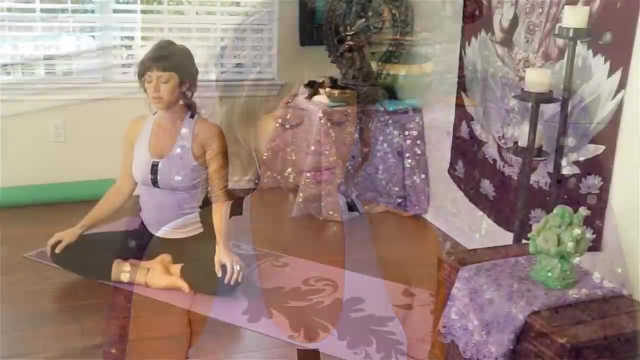 Take a moment to rest here And, as you are ready to come to a seat, use your top hand to press yourself open the way up. See if you can keep your eyes closed so you stay in this quiet and meditative space. Find yourself in a comfortable seated position and let your 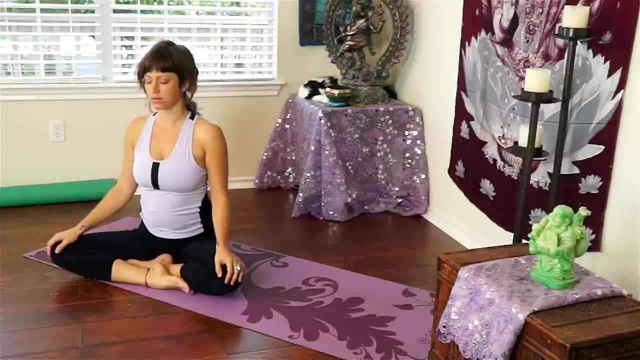 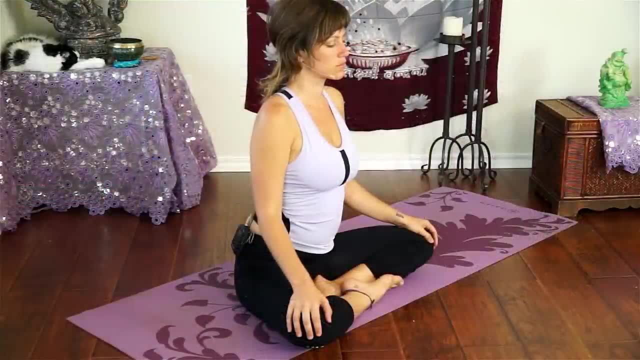 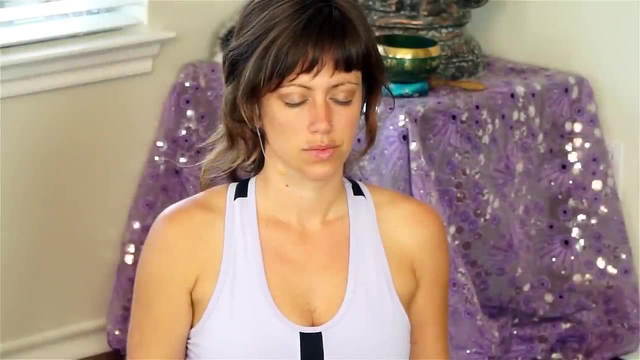 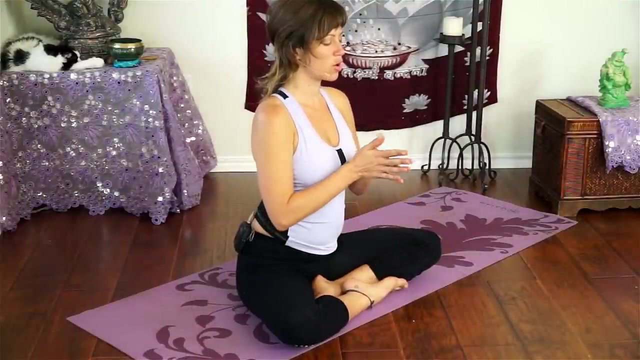 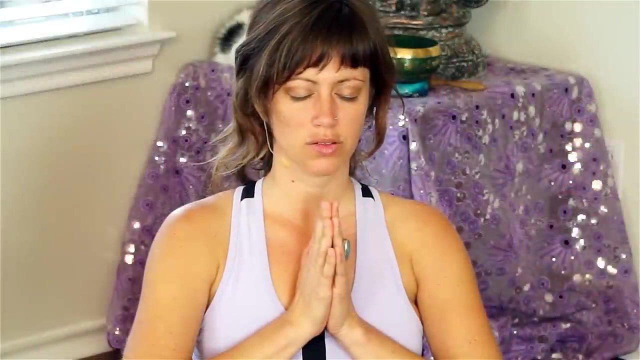 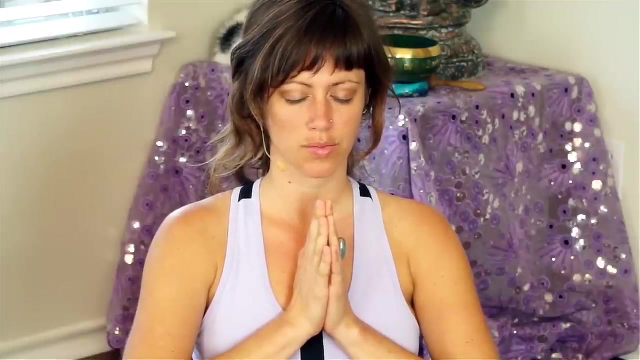 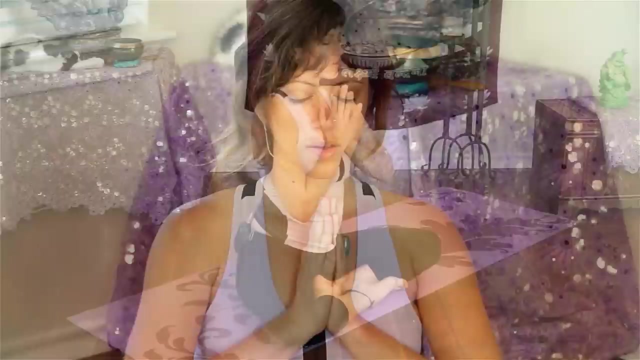 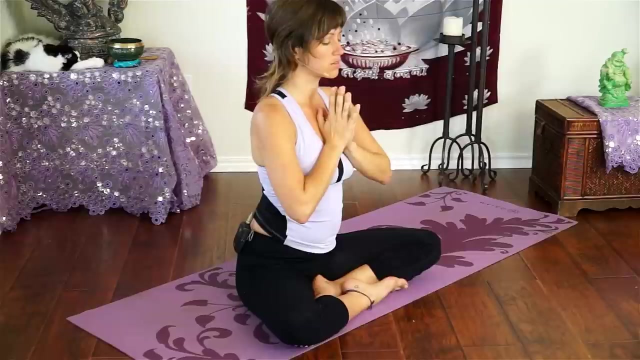 hands rest on your knees, Slowly, bring your hands to prayer at your heart, pressing your palms together, And take this moment to thank yourself for using this time to take care of you. So often in our lives we can become distracted by taking care of so many other people and things. 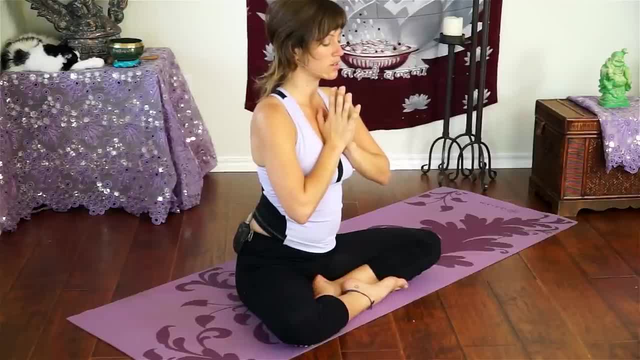 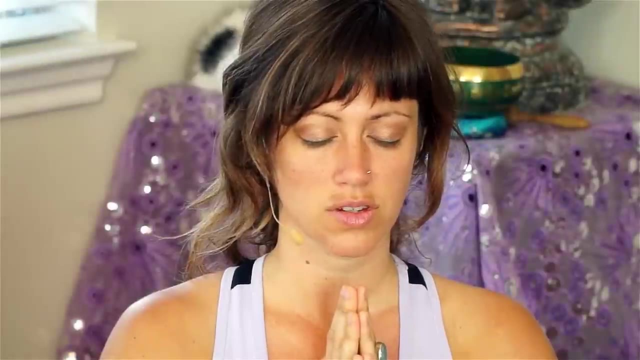 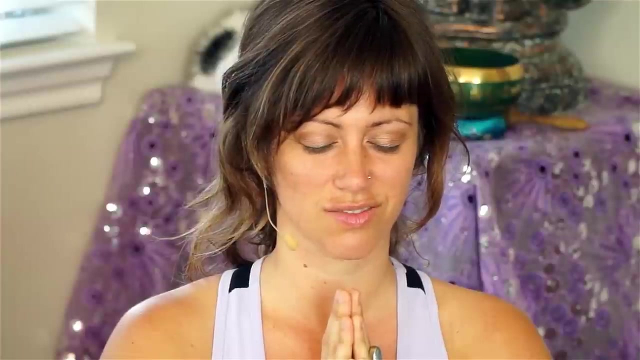 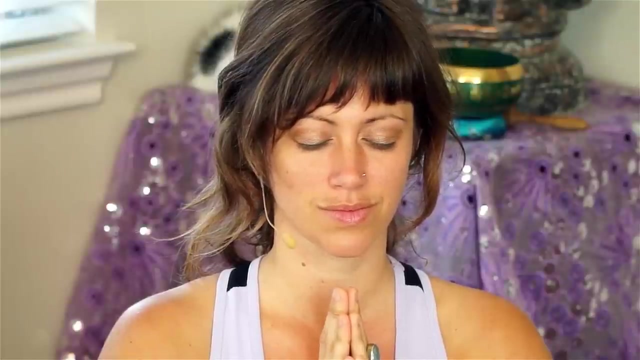 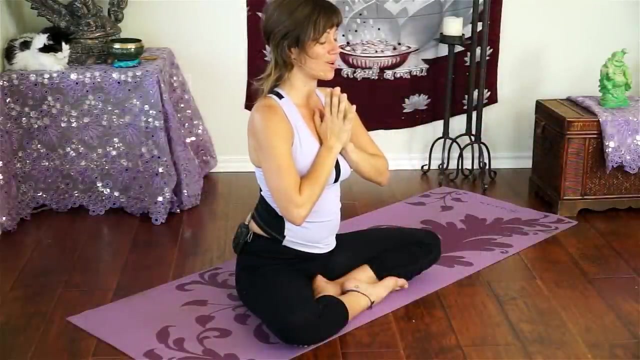 It's amazing how easily and how quickly we forsake ourselves. So just thank yourself right now for giving yourself this attention. You deserve it. Thank yourself for giving yourself this attention. You deserve it, And take this time to say you're welcome. 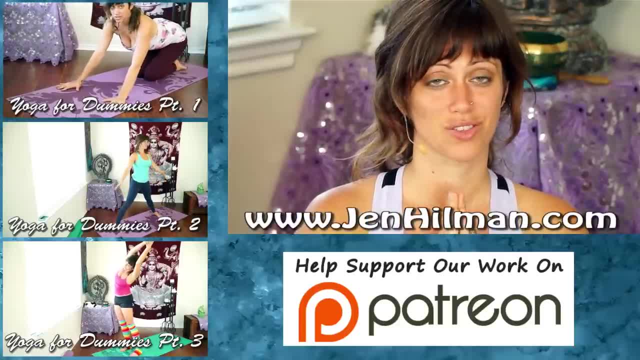 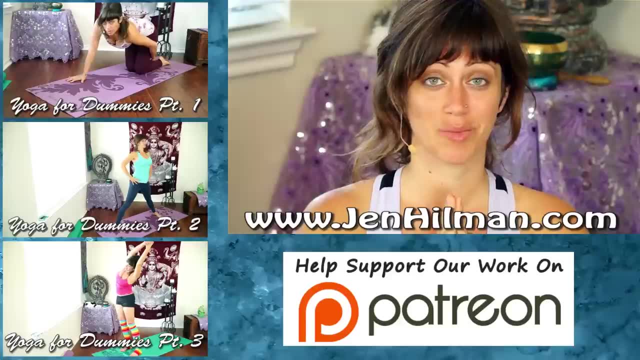 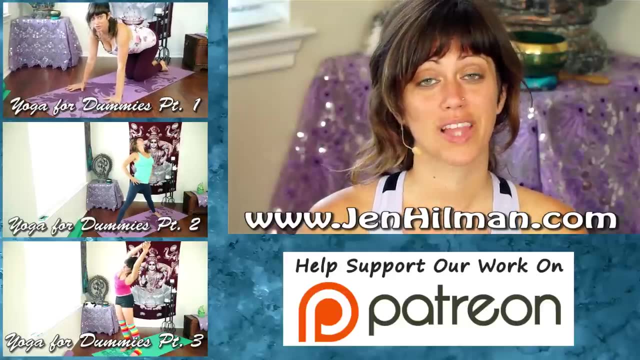 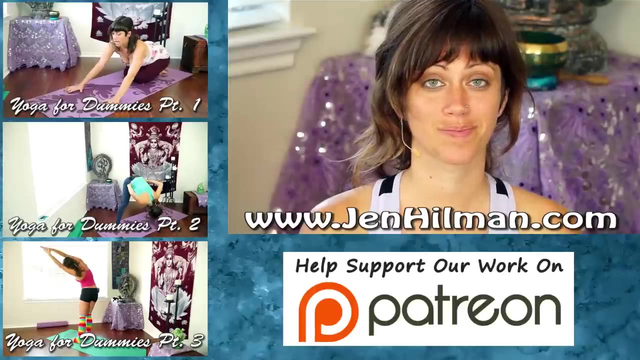 And I also would like to thank you so much for sharing in this practice with me. Thank you for letting me guide you and share my passion with you. If you'd like to learn more about me, visit my website, JenHillmancom and subscribe to. 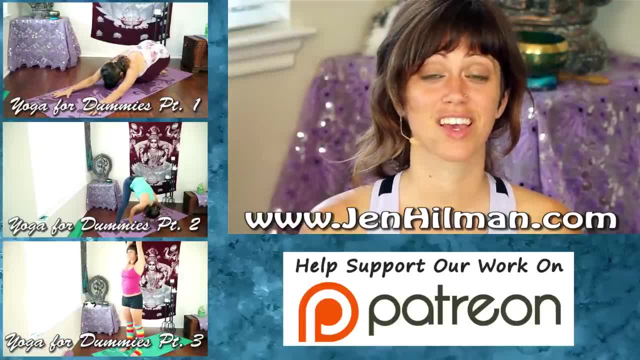 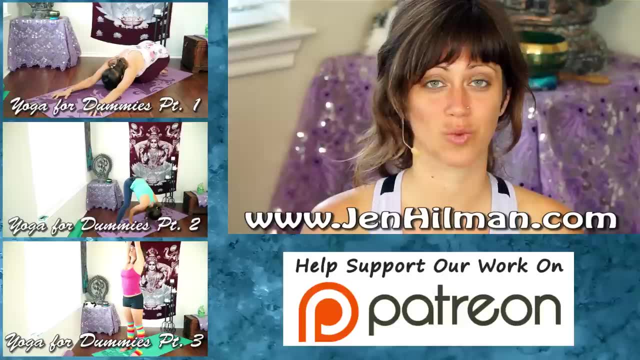 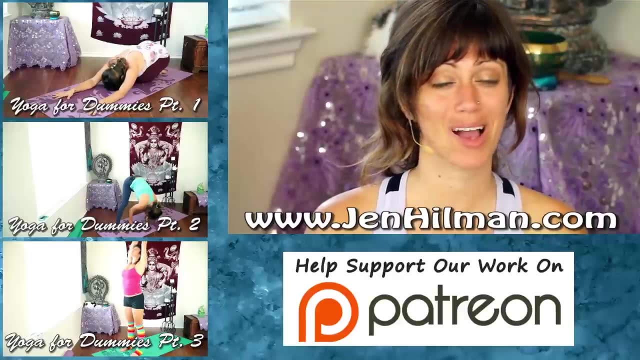 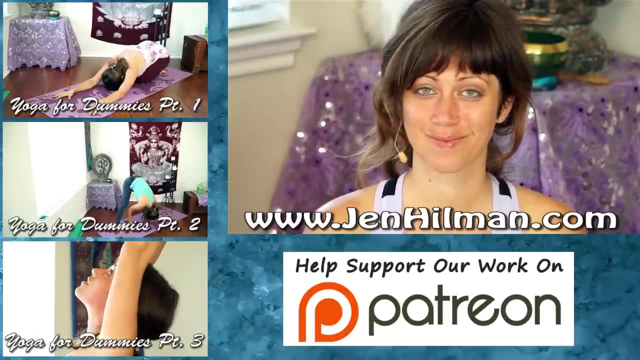 the Psyche Truth channel, where you can have access to all of my yoga for beginners videos and lots more fitness and wellness videos for your body. Don't forget to favorite this video so you can come back and practice anytime you need to relax. You deserve it, don't forget.